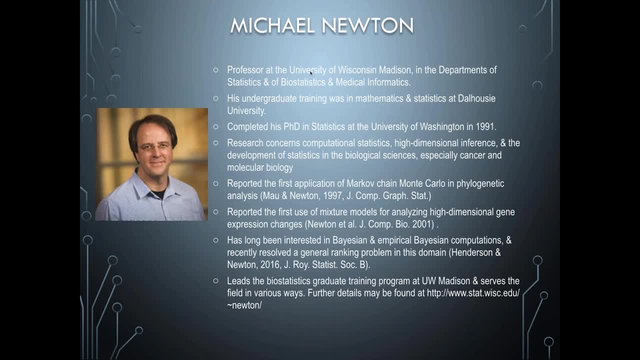 Advanced site: good, great. Dr Noonan is an associate director of the Center for Predictive Computational Phenotyping, CPCP, one of the national BDTK centers of excellence. Dr Noonan has led many novel applications of statistical techniques and algorithms on biomedical big data, For instance. 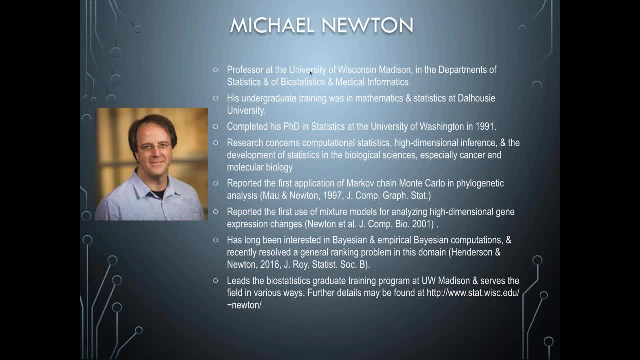 he was the first to use Markov chain, multi-carlo and phylogenetic analysis, as well as the use of mixed models for analyzing high-dimensional gene expression changes. A long-standing interest of Professor Noonan is that he is a professor of statistics and biostatistics at the University. 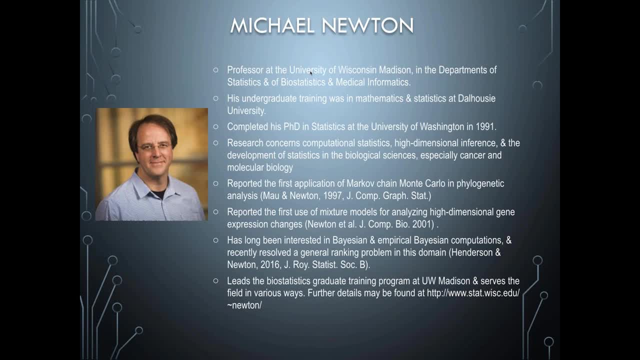 of Wisconsin-Madison and is in the area of Bayesian and empirical Bayesian computations. He will be talking to us today about Bayesian inference methods, So please join me in welcoming Dr Noonan this morning. Michael, thank you for joining us. The floor is yours. 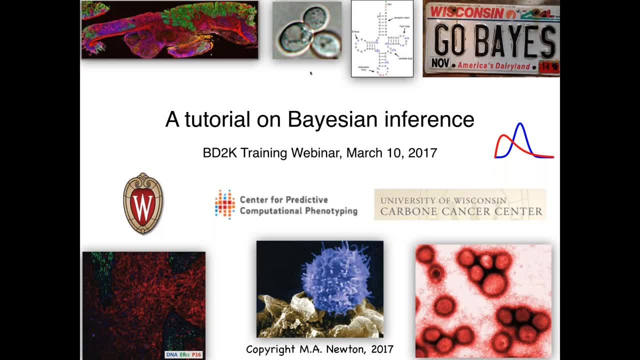 Thank you, Alex. Well, hello everybody. It's great to be here. Thanks for tuning in. I do hope you find something useful in today's webinar. So the pics on this first slide signify some projects and activities that I've been involved. 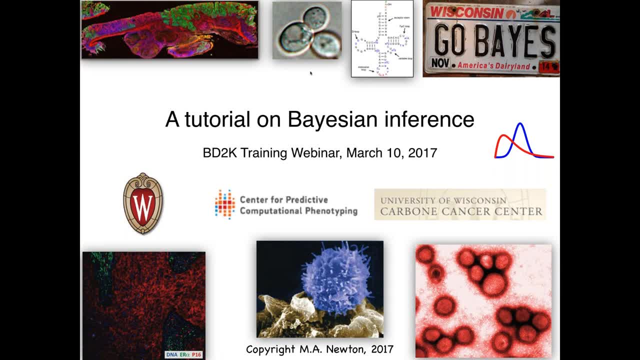 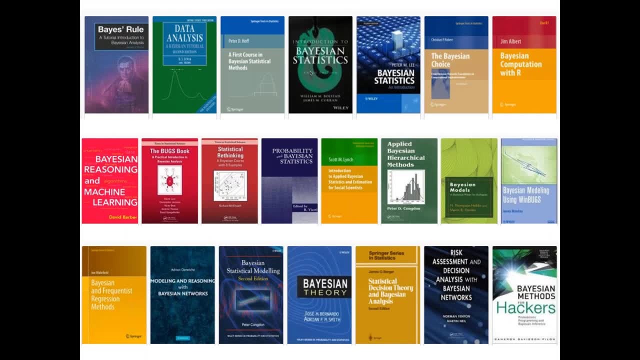 in in my own work And they may show up in examples as we go through today. Well, Bayesian inference is a big deal. Lots of researchers have thought a lot about it and how it can be used to advantage in data analysis. There are a few books on the topic. 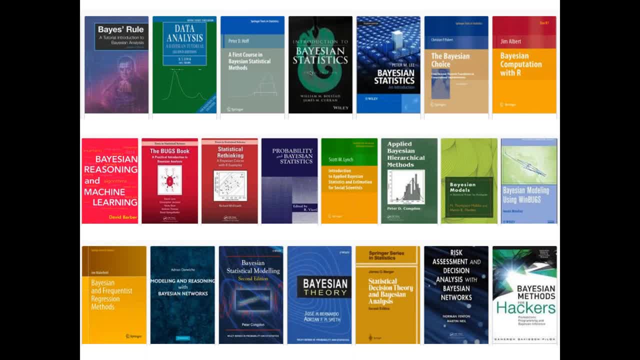 and I encourage you to take a closer look. My goal today is to be sort of a cheerleader for Bayesian methods, pointing out some of their basic features and also some opportunities in this new world of data science. But in addition to my job, there's 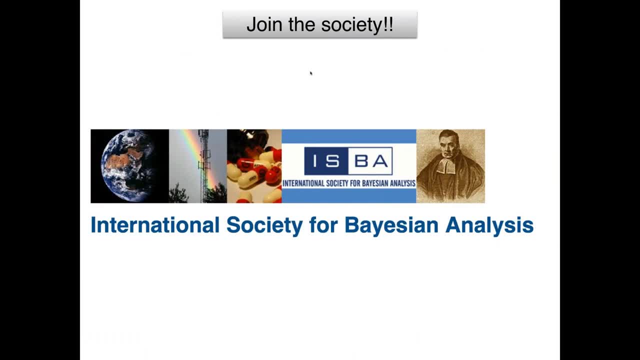 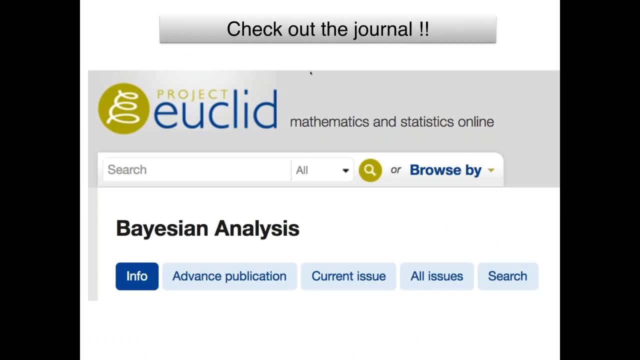 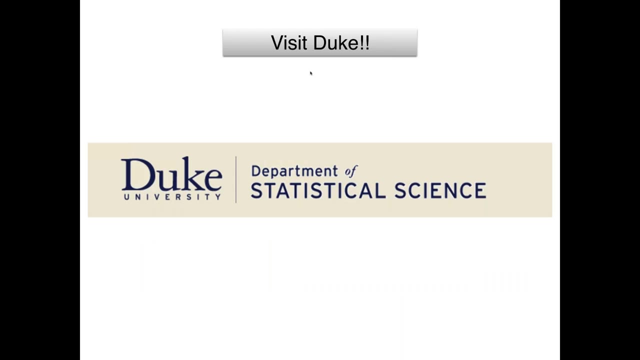 some things for you to do too. You can join the Society for Bayesian Analysis. You can check out the American Statistical Association section. You can check out online the journal Bayesian Analysis. You could, in fact visit Duke University, where it's one of the strong centers for Bayesian inference. 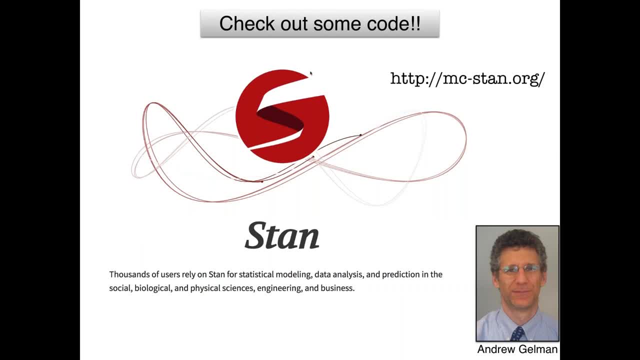 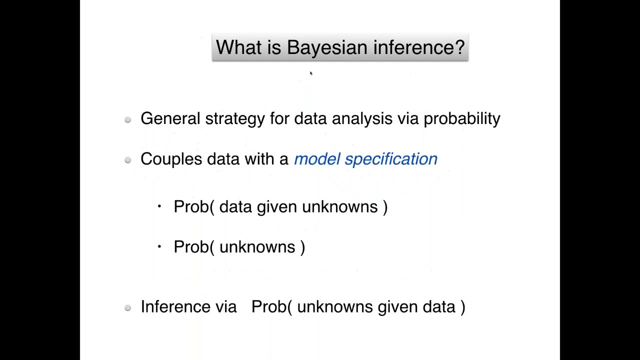 and research in these techniques. You could check out some code. Andrew Galman's originated this terrific code project called STAN that delivers some really useful software techniques for deploying Bayesian analysis. So that's some of the things you can do. I'm going to just give you a bit of an overview of what 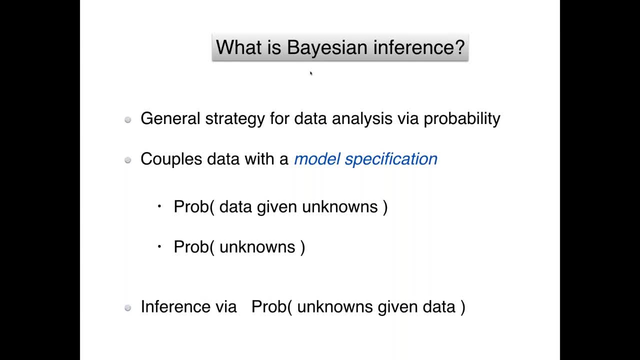 Bayesian analysis is some of the key features about it and how it goes in some examples. So it's a general strategy for data analysis based on probability And the key thing about it is it couples data with some kind of model specification and that model 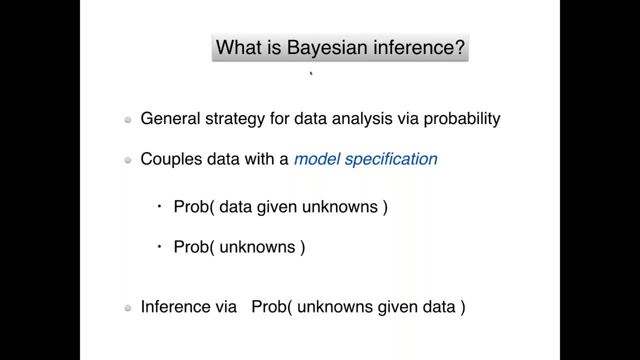 specification has two features. It's got a probability structure for the data themselves, given unknown things. This reflects kind of the central dogma of statistics that all data sets are the realization of some random process And encoding that in probability is kind of central. 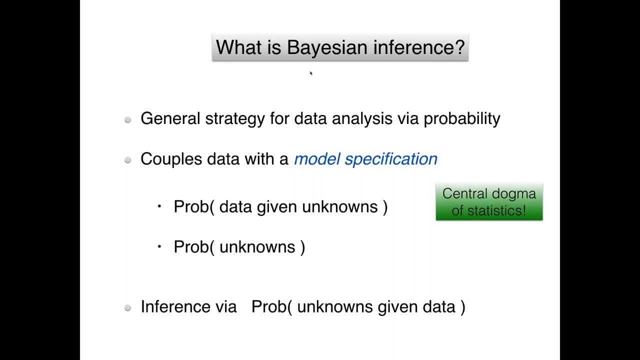 But then the second part of it has to do with all the unknown parameters, say, And there's some probability structure on that too. that's a special part of Bayesian analysis. It essentially expands the domain of probability to be a general measure. 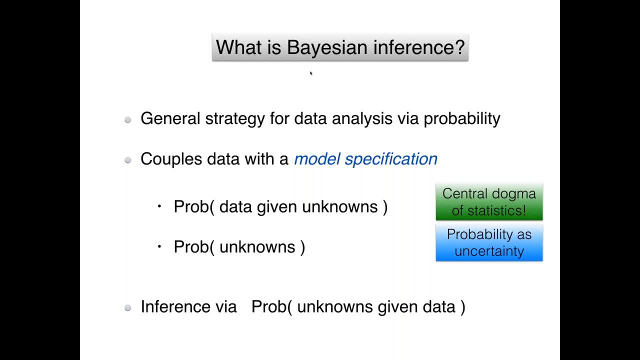 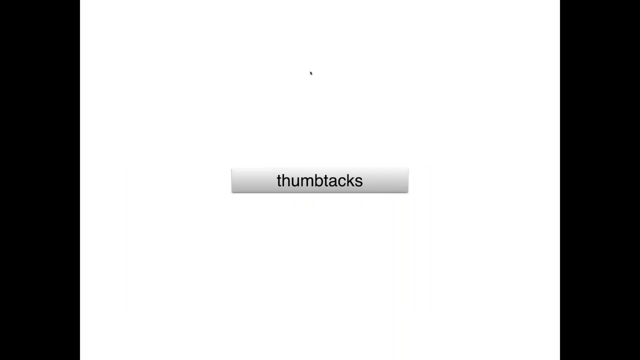 It's a measure of uncertainty And then inference about what we don't know, given what we know proceeds using the rules of probability. OK, well, I'm going to talk about a few sort of relevant examples, But I wanted to start with a kind of irrelevant example. 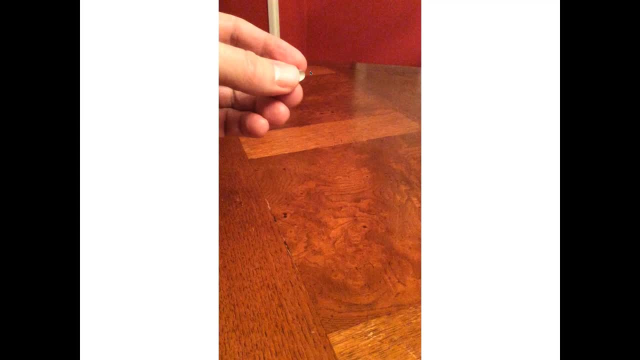 but it's still pedagogically interesting about thumbtacks. So here's a little video. I'm doing an experiment to collect some data. I'm tossing a thumbtack And notice that I tossed that tack and it landed with its point facing down. 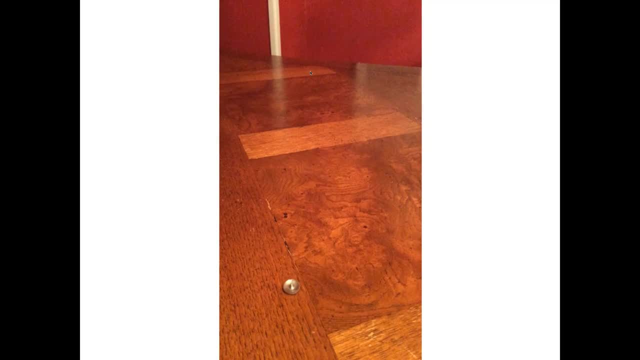 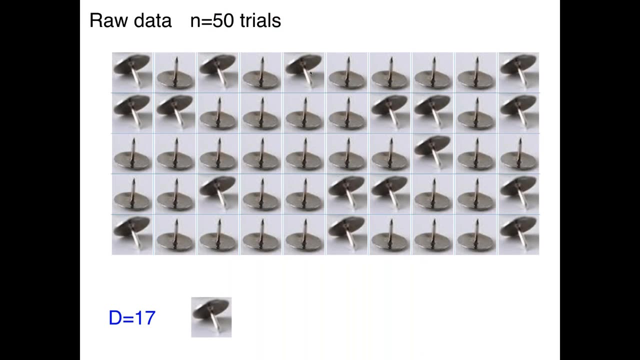 I replicated that experiment again and I tossed the tack and it happened to land with its point facing up, And this was the beginning of a longer experiment that I did with 50 trials, the outcomes of which, a full data set, is shown here. 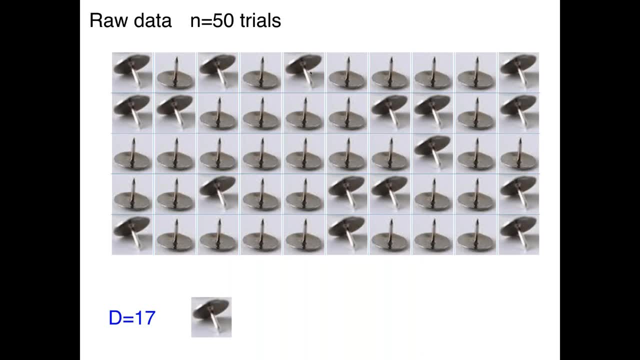 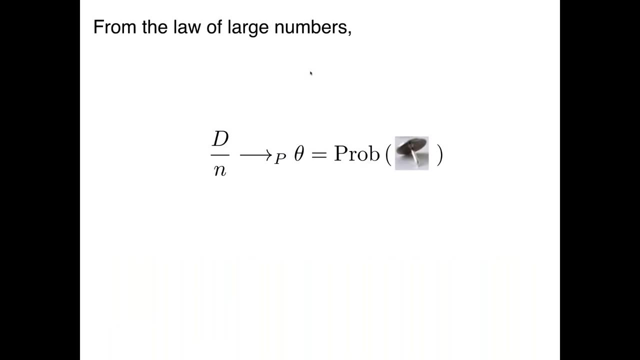 I got in my 50 trials it turned out 17 times that the tack landed with its top side, with its point facing down. Now we know from the large numbers that the relative frequency at which the tack lands with its tip point facing down 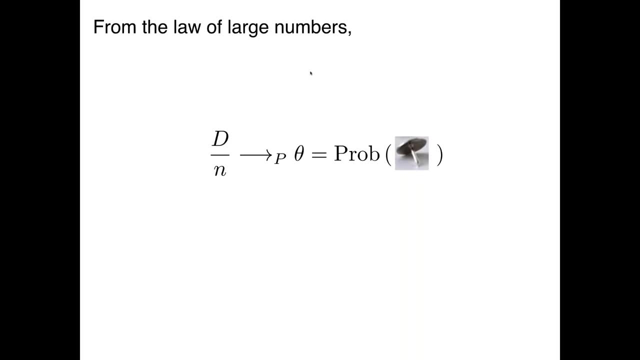 that d over n, that relative frequency is well. it's a random variable, for one thing, but also it stabilizes In the long run. if I were to have continued the experiment tossing tacks indefinitely, it would converge to something. 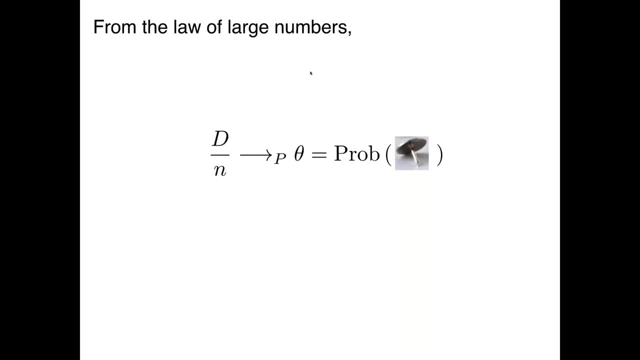 we'll call theta the long-run relative frequency of times that the tack lands with its head pointing down, And that's a parameter of the system, a property of the tack in the experimental system, and it's an unknown underlying parameter underneath the data set. 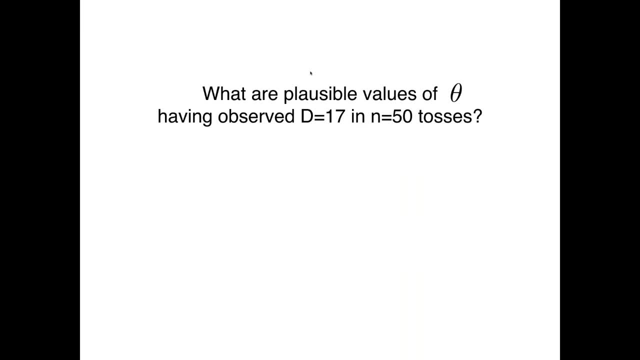 So we could of course estimate that unknown theta with 17 out of 50, 34%. But at issue really in our focus are asking more general inference questions such as what are plausible values of that parameter, having observed 17 tack points down in 50 tests? 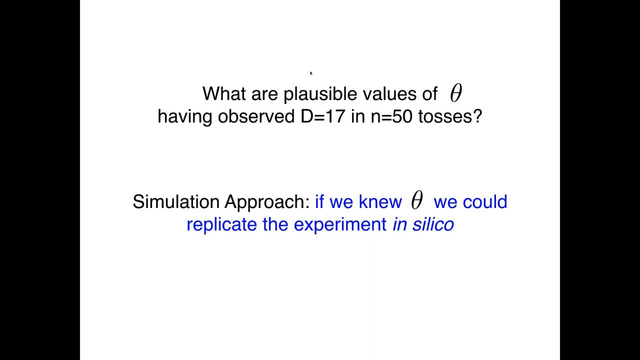 And rather than go through the math of it, I just wanted to present this, answer this question, as Aysen would answer, but through a simulation. So in this first part of the simulation, suppose we happen to know this long-run relative frequency. 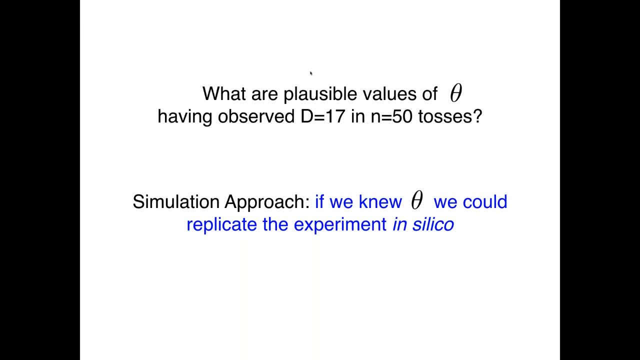 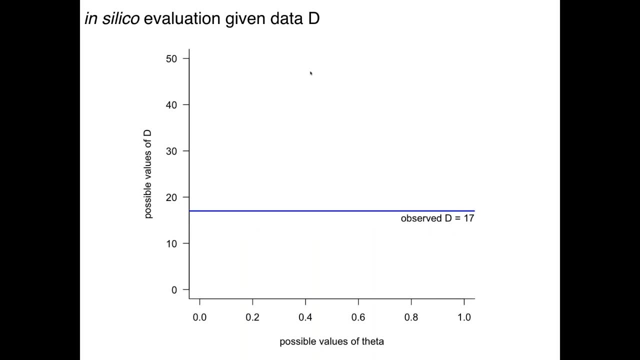 theta. If we did, we could surely run the experiment in the computer and replicate it. So this little panel is sort of set up to understand replications of this little tack tossing experiment. I've got possible values of theta on the horizontal and I've got possible values of theta on the vertical. 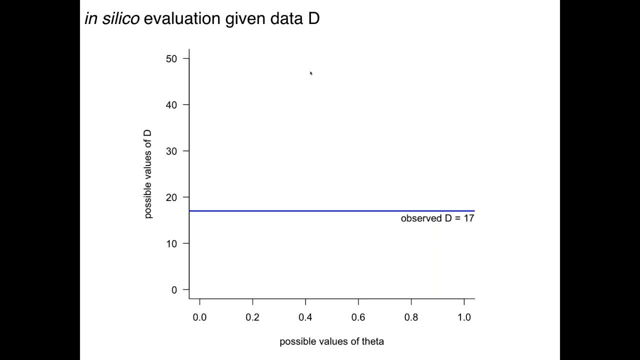 And the ability to do that is. I'm going to take the observed value of the data 17 times that the tack face, pointing down out of 50 trials. Now look at the little code chunk up in the upper right here. This is my in silico experiment. 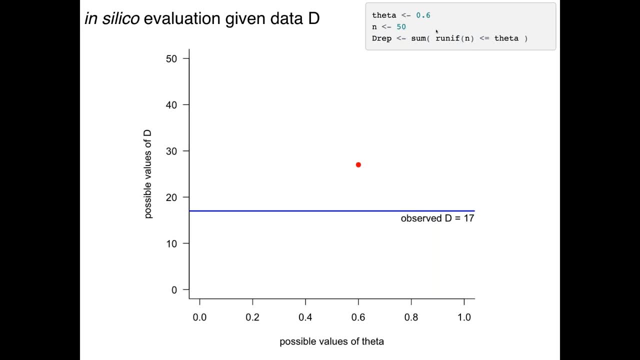 I could fix theta, for instance, if I knew it, at, say, 60%, and set up this little code which just is a way of using random numbers, pseudo-random numbers- in the computer to simulate the tack tossing without actually tossing the tack 50 times. 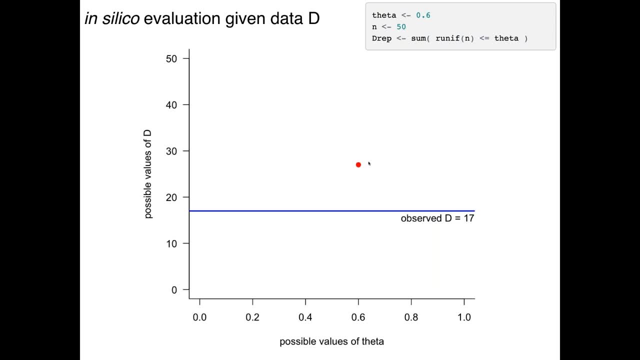 But this is a replicate of that- if I knew that long-run relative frequency- And I happen when I do that to get about 26.. Now, since it's a simple bit of code, I can repeat it. Obviously, I can repeat it. 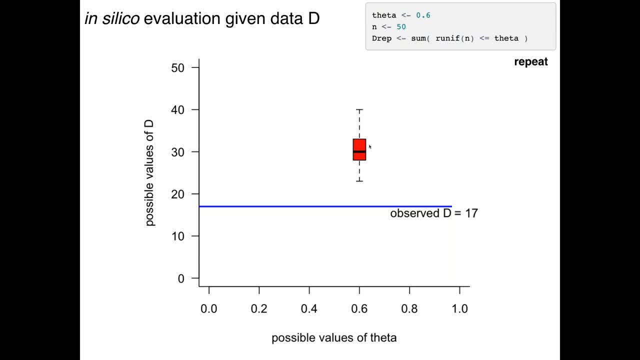 And look, I did it about 1,000 times And this represents the so-called sampling distribution. You'll recognize the binomial sampling distribution of the relative of the values, of the number of point down tacks: out of 50, centered around 60% of 50,, around 30,. 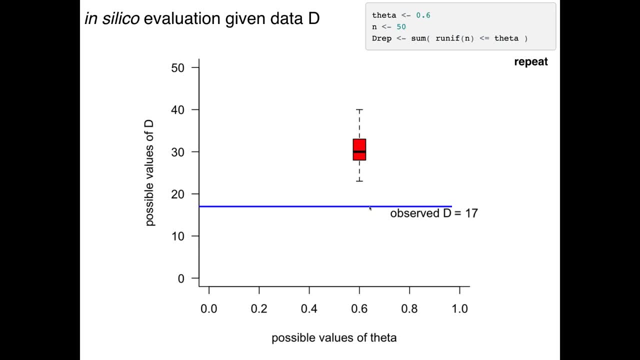 but with some fluctuation, And notice that the value, The observed value of 17, doesn't look very plausible for that data set, And that's basically a problem with this little simulation. I've had to pretend I know the value of this unknown parameter. 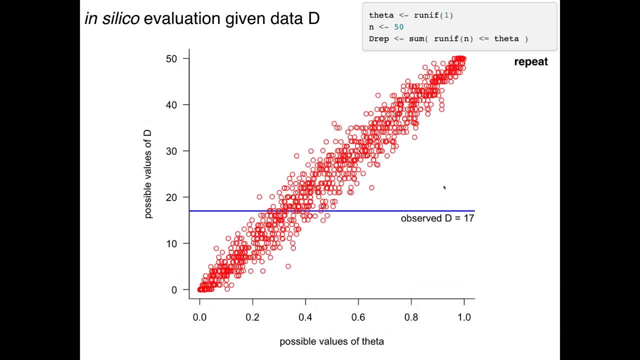 when in fact I don't Now as I do that simulation, I could just change it a little bit. If you look up here, as I imagine, what data I might have happened I might have gotten, let me also vary the value of the parameter theta. 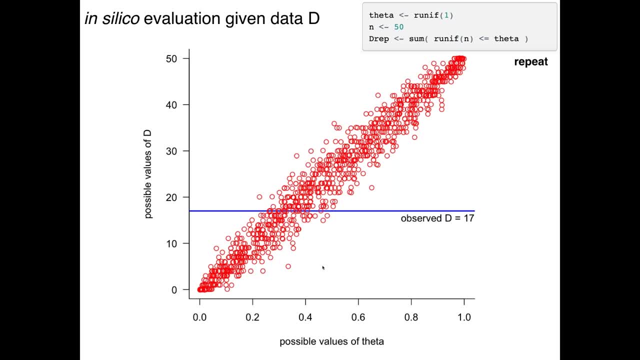 I just grab a uniformly distributed theta every time And on that uniformly distributed theta, then go ahead and simulate my outcome of my experiment. This is what you get if you do it about 1,000 times. Now what's round and gray? there is these. 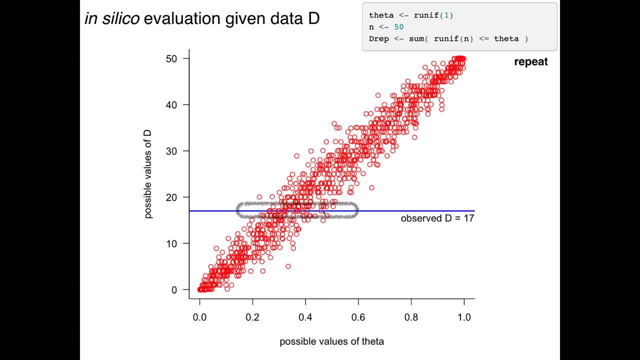 are hypothetical repetitions of the experiment that I've set up in this two-stage experiment, where the simulated data are actually exactly the same as the data that I happen to see in my real experiment. So surely those values of those parameters that gave rise to those simulated data, 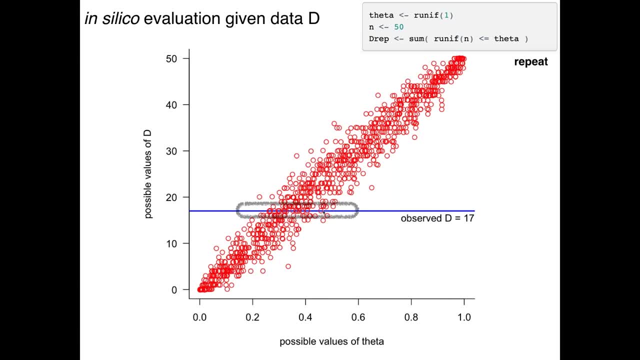 must be plausible because in light of the data that I saw, they could easily have given rise to the same data as we saw in the simulation. So that is the essence of what Bayesian analysis is: It's looking at the distribution of those theta values. 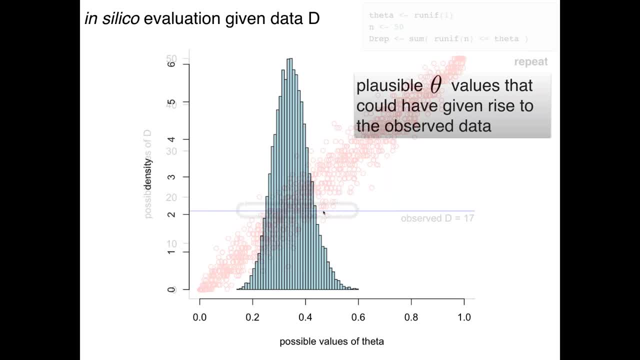 Now we've conditioned effectively on that 17, and we can project down onto the theta axis right now, And so I've just taken this, boosted the simulation and I'm going to license, size up a bit. But this is the distribution of the thetas. 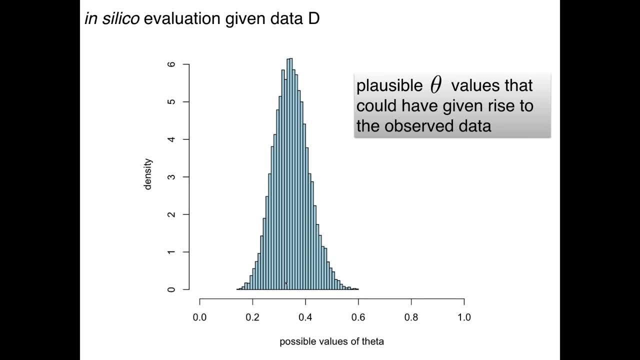 that came out of this experiment, where I first simulate theta and then I get simulated data given theta, But then I keep a track of the thetas that match my observed data. These are certainly plausible values. Well, indeed, mathematically we can work out. 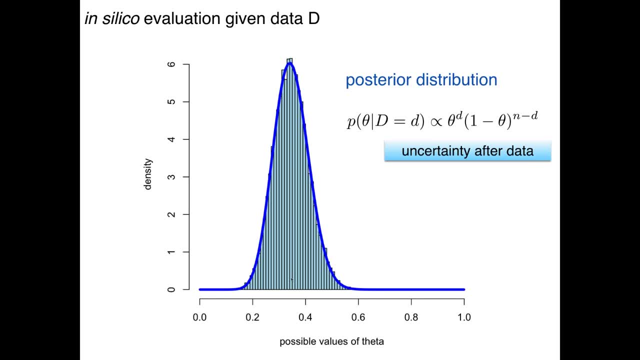 the formula for that curve- It's known as the posterior distribution, Functional form is known And it expresses a kind of uncertainty in the value of theta that would have generated the data we saw. But the uncertainty is that it's not going to be expressed after the data have been seen. 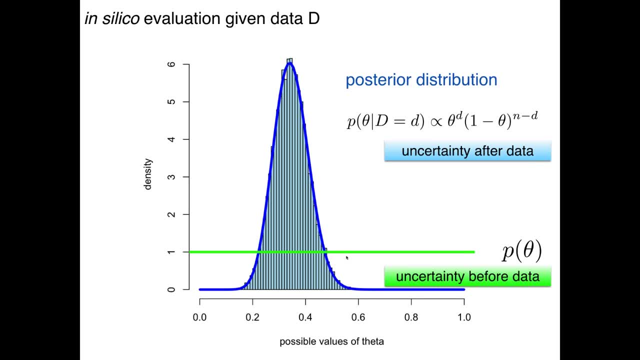 That's to contrast it with the uncertainty that we expressed in this little simulation before the data we're seeing. Remember that RUNF chunk of code which said what the theta values are before What theta values I'm considering is relevant, in advance of having seen the data. 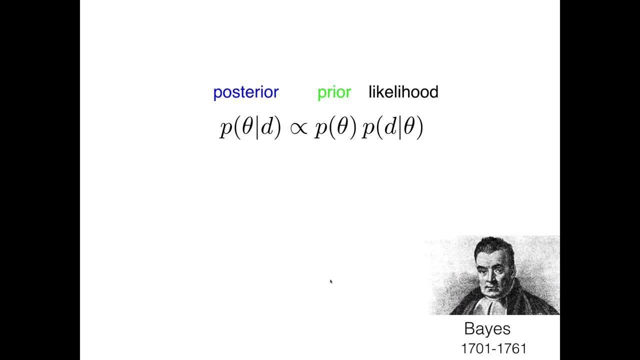 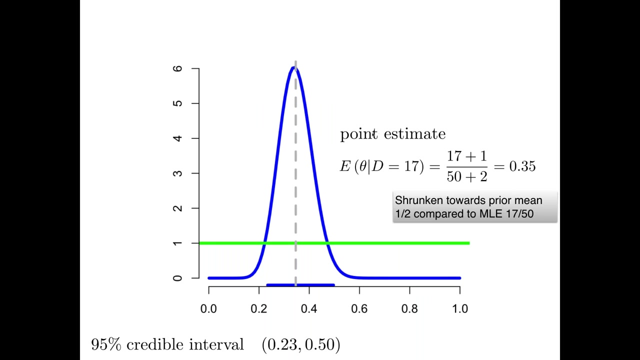 And this connection, the connection, the famous formula that the posterior is proportional to the prior times, the likelihood that's likely now coming from the binomial model. In our case it goes way back to Thomas Bayes himself. Now, looking at that functional form, this is the this thing. 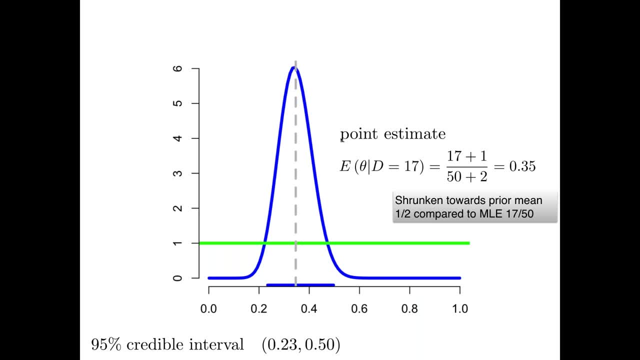 this beast is the object that is critical for inference. So we could take a- we don't know that- theta. We have a summary of our uncertainty about it. If we take the center value, the mean of that distribution, its expected value, that could serve as a point estimate. 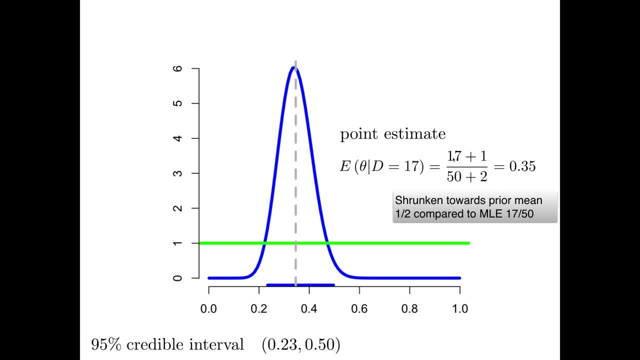 And it happens in this case that the balance point of the distribution is a little different. It's a little bit different than the what you would think of as the natural estimator- 17 over 50.. It's a little bit modified. It's, as we say, shrunken towards the prior mean. 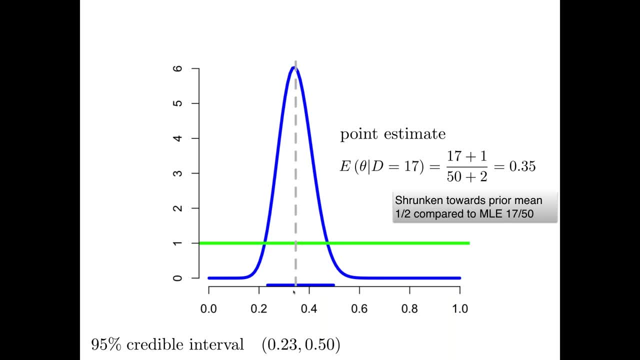 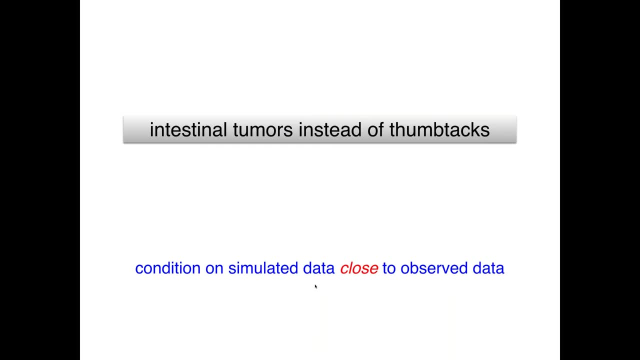 which is a half compared to the MLA. We could also get an interval that contains a certain amount of that posterior problem. So that's how it would go in this little toy example. Now let's take a second, less toy example: intestinal tumors. 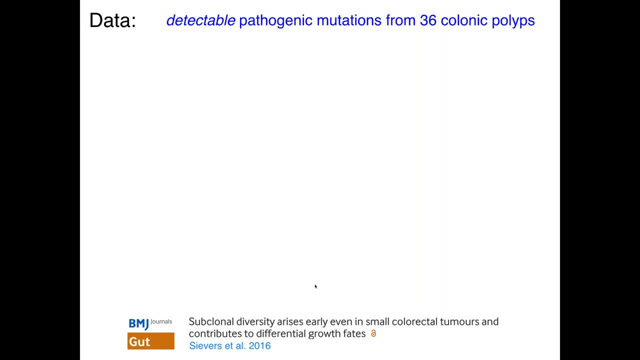 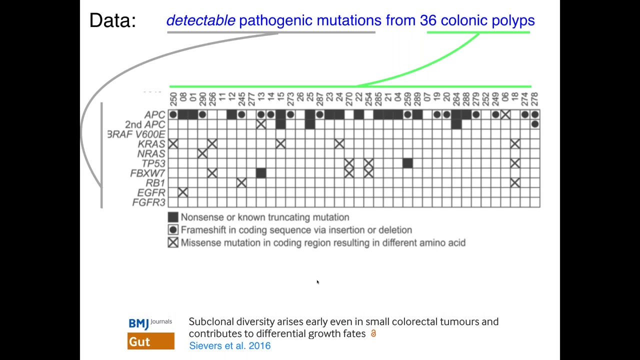 Now, here the data aren't tied to outcomes of attack throwing experiment, But they're outcomes of looking inside the DNA of polyps that were found during colonoscopy of men. in a study, Detectable pathogenic mutations from 36 colonic polyps. 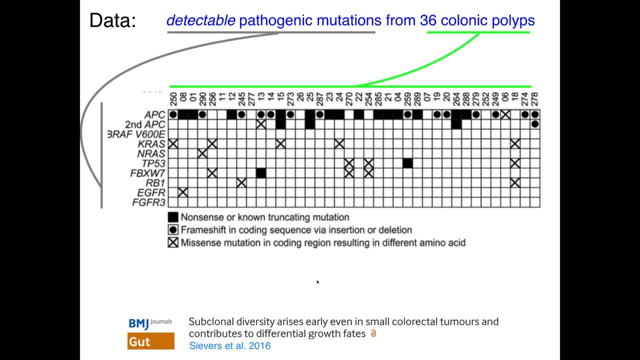 Here's the data here: The horizontal corresponds to the 36 different subjects in the study. The vertical are the rows correspond to different pathogenic mutations that were measured, different genes that are known to be critically involved in the development of colon cancer. 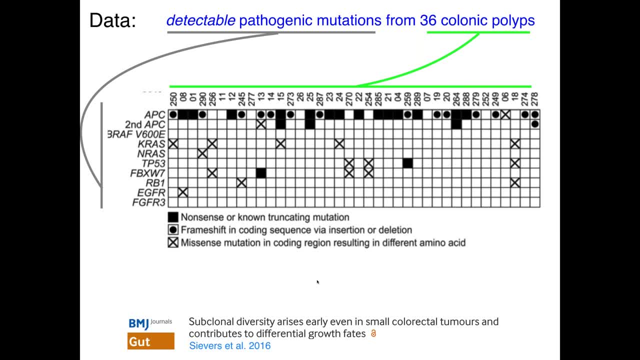 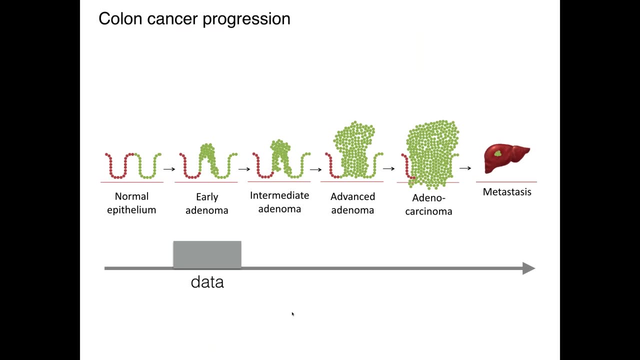 That's the data. These are detectable, So they have to have appeared at a sufficiently high frequency in the sequencing of the tumor. This comes from a recent publication by Chelsea Sievers and Rich Halberg's group here at Madison. Okay, Now I have to give before I tell a bit about the model. 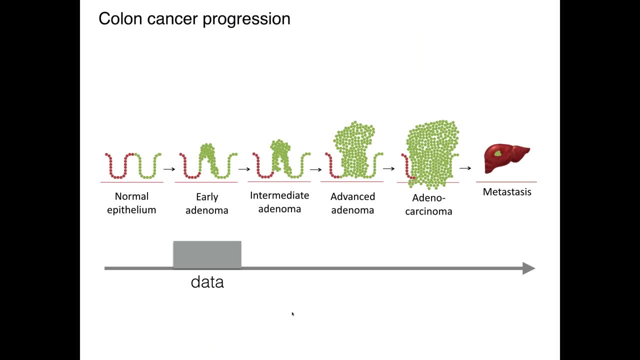 I have to say something about colon cancer progression. This little cartoon on the left shows the wall, just a tiny segment of the wall of the intestinal epithelium, And the green piece here has been converted. It's initiated to be it's non-normal. 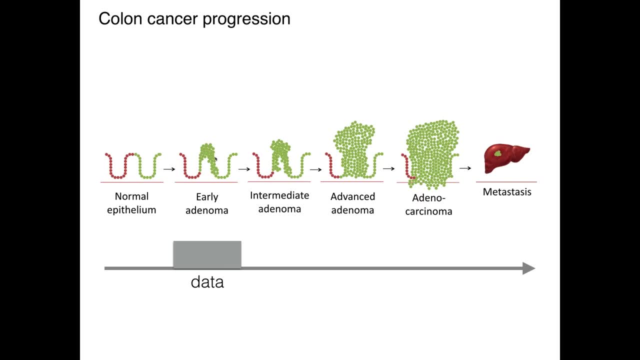 and it's starting to become cancerous. The polyps are essentially at this stage, The data is coming at this stage, Abnormal growth outside of this structure here And eventually, if things go wrong, you'll get a cancer. But the data that we're talking about are data. 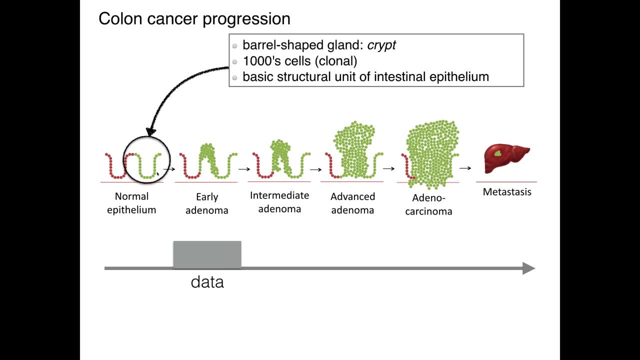 from early adenoma stage. I also want to point out a basic structural unit of the intestinal wall that's expressed here in cross-section in this cartoon. The intestinal wall is made up of these millions, I guess, of these barrel-shaped glands, called crypts. 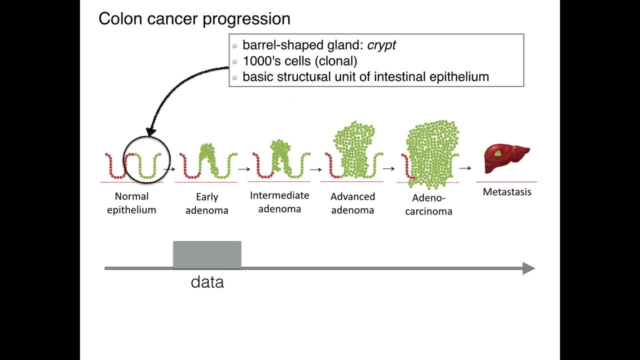 They're actually thousands of cells, not just a handful of cells here, And they're clonal. So essentially they all come from stem cells at the bottom of this space that they have. They're from a single lineage. That's going to be important in something I'll say later. 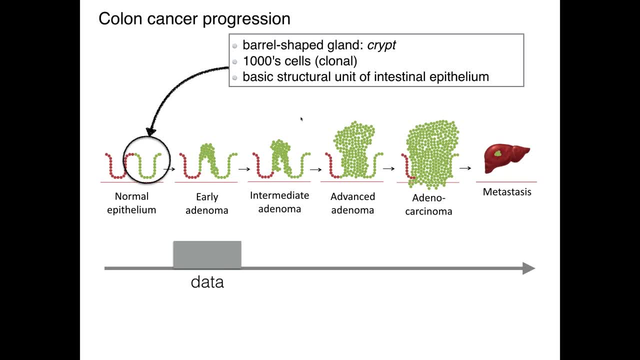 They are from a single lineage And they are the basic structural unit of the intestine, like I said. And also tumors, when they start, are initially adenomas. They emerge out of these crypts and they start to grow. There's a whole bunch of interesting things about crypt. 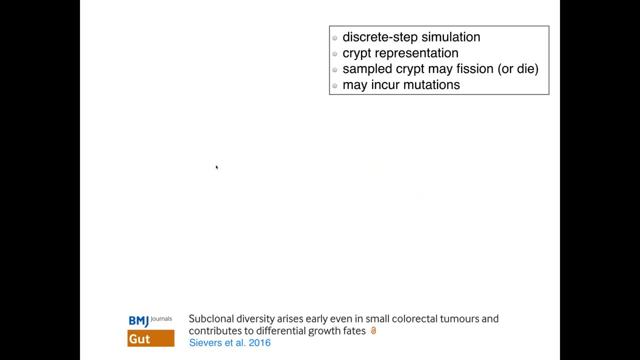 biology, I won't say, but the crypt itself is going to be an important thing for my story. Okay, So previously we tossed tax in silico, But now, instead of tossing tax in silico, I'm going to do a simulation of tumor growth. 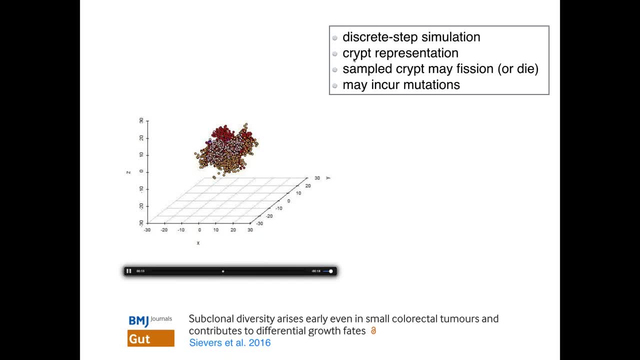 It's a discrete-step simulation. It's not cells that are shown here, but actually crypts that precede This, evolved by a certain stochastic model that you can read about in the paper. Essentially, crypts may fission. They can turn into multiple crypts. 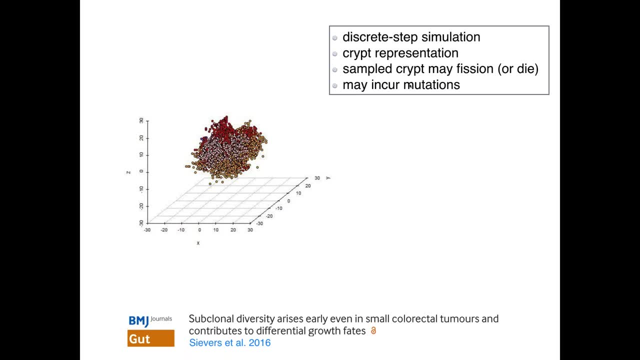 or they could potentially die, And also the crypts. these clonal bodies may incur certain mutations as they go along The colors that you may be able to see here there's different colors corresponding to different mutations that have occurred and then grown out. 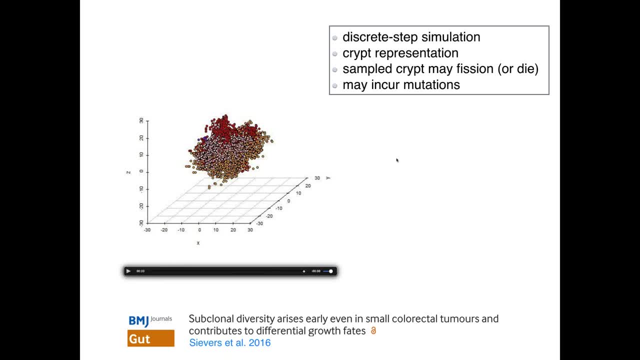 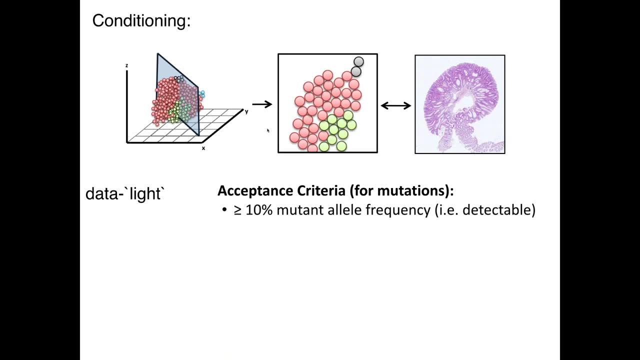 So this is an interesting thing. So it's not tossing a tax, but it's growing a tumor. Now, well, what did sievers do? They would simulate these tumors and then they'd mimic the sampling process. They did an in-silico section of the tumor. 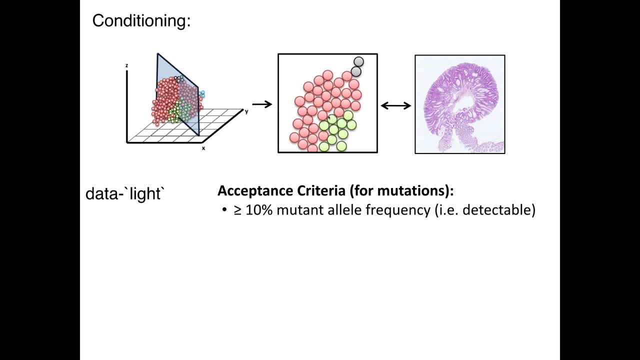 looked at the crypts inside. Basically, we're trying to match what they observed here with our observed data on the 36.. Now in the sievers paper they do something very light. Instead of conditioning on all 36, they just ask a very, very simple question. 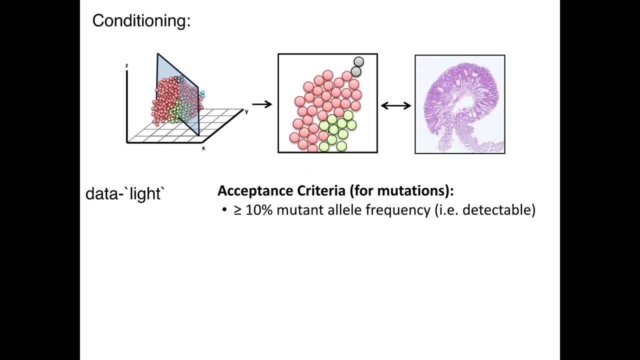 It's a little bit different than conditioning on all the data. They just ask: at the level of a mutation that you would see in here, does the frequency at which that mutation occur? does it exist at a sufficiently high frequency to be detected by the next-generation sequencing technology that's used? 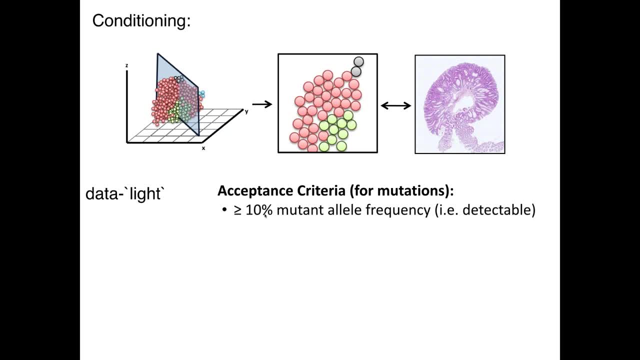 And their lower threshold was that the mutant frequency had to be bigger than 10% in order for the sequencing to observe. Is it a detectable mutation? Now, ideally, in fact, we would simulate not just one tumor up to check for its mutation, but we would simulate a sample. 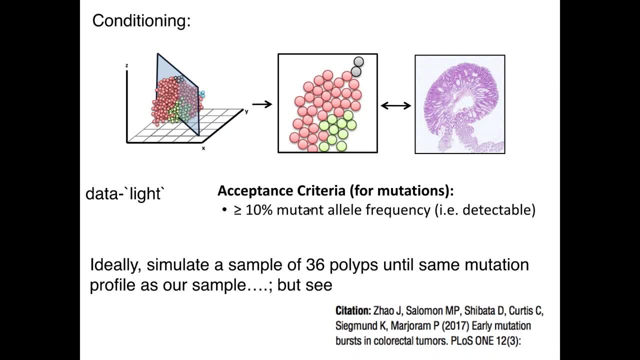 of these polyps or tumors And you'd wait and you'd see if the mutation profile and slices of these things matched our observed sample. We don't do that, Sievers didn't do that, But I just point the interest of the observers to this paper. 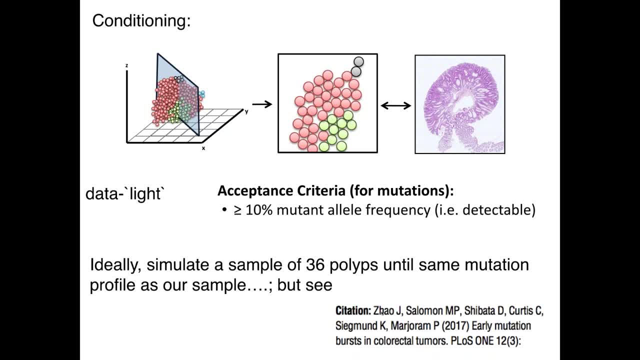 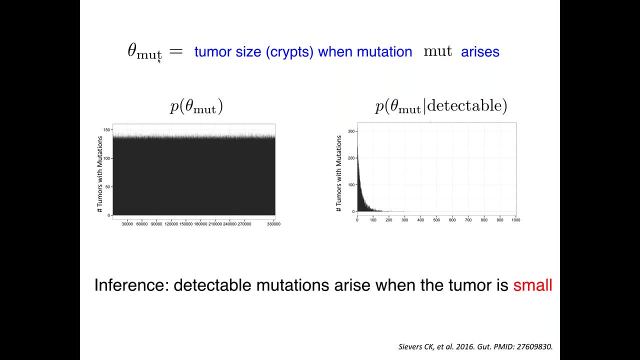 that just came out earlier this week by Marjoram's group that does essentially that. It's just a kind of a calculation. In any case, in the simple calculation that we're talking about, where we simulate up instead of tossing a tack, 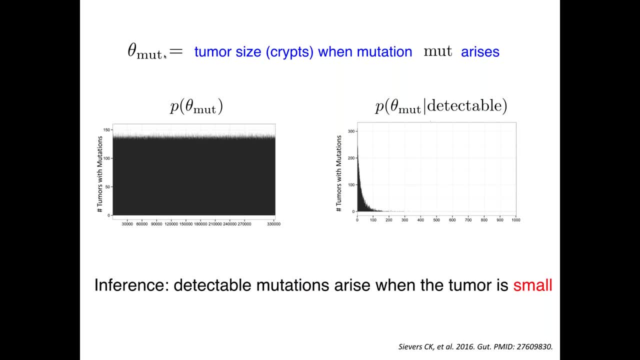 we're simulating up a tumor that's growing in the intestine through a stochastic model of how tumors might grow and we look at a mutation that's shown up at the time that we observe the tumor. the quantity of interest in Sievers' paper. 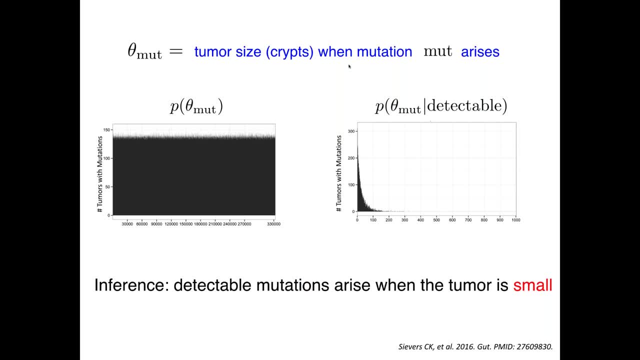 was the size of the tumor in CRIPS when the mutation that we're looking at happened to have emerged. So when we see it at observation time we get to see a mutation at some frequency, But that mutation must have emerged in the tumor growth. 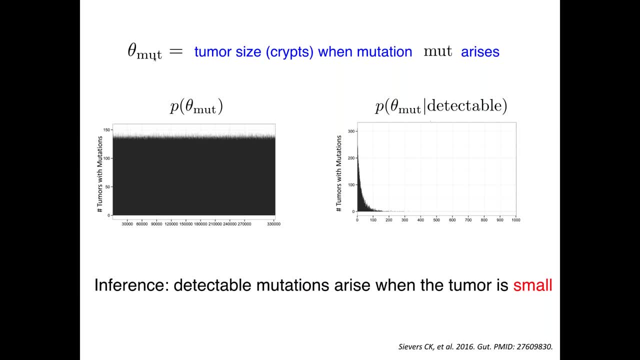 sometime before we got to observe it. That time isn't known to the observer. That's the parameter theta sub mu, And the simulation is rigged up so that these tumor mutations can emerge at any time along the – they can emerge at any time in the sense of any size that the tumor is as it's growing. 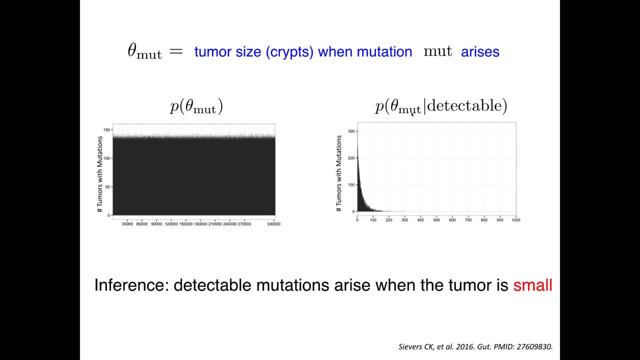 But if we condition on the data, so to speak, that we condition on the fact that the mutation is actually – exists at sufficiently high frequency to be detectable when we measure it, then we get a posterior distribution of the size of the tumor when that mutation arose. 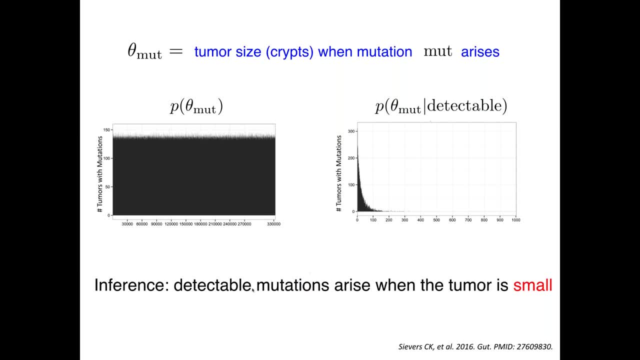 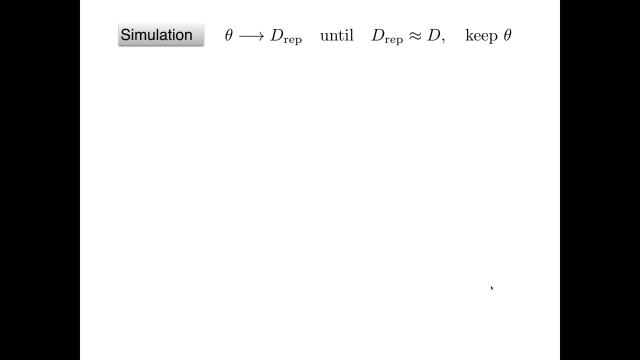 And looking at these kind of distributions tells us that these detectable mutations must have arisen when the tumor was actually quite small, And you can get specific inferences about that. So that's an interesting variation of the simulation story where, instead of simulating tax, we're simulating tumors. 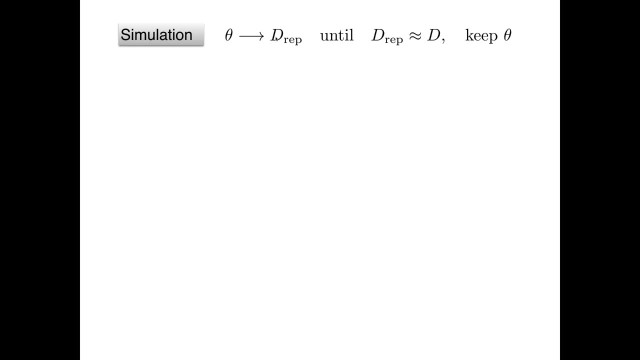 But the same story: you simulate unknown things, data, simulated data, until that data is equal, or approximately equal, to the observed data that you have and you keep a track of the quantity theta that corresponds to it. This simulation view of the Bayesian inference was one of the number. 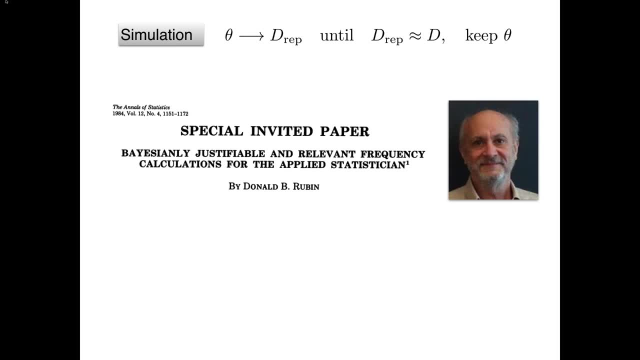 of terrific insights made by Don Rubin in his paper that I recommend everybody on, And I think it's really interesting to see the frequency calculations that are relevant for Bayesian analysts. That's also the basis of what people now call approximate Bayesian computation. That's especially useful in situations where likelihood 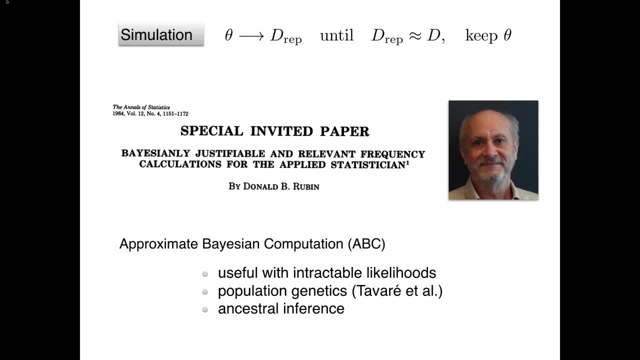 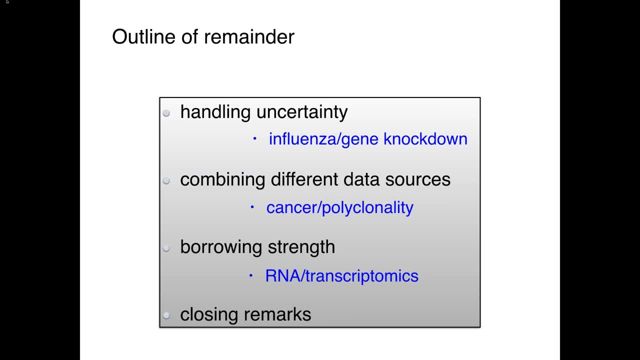 functions are intractable, such as in population genetics or in other forms of ancestral inference. Okay, so that's just a little supposed to whet your appetite about Bayes. from a simulation perspective, I want to talk about three main features of Bayes. 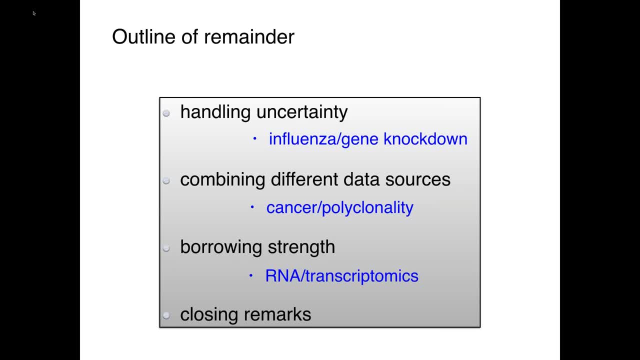 Going forward now with the rest of my time. So I want to talk about three basic things: handling uncertainty, combining different data sources and borrowing strength, And I'll use three different case study examples to illustrate these features of Bayesian inference. So let's go forward. 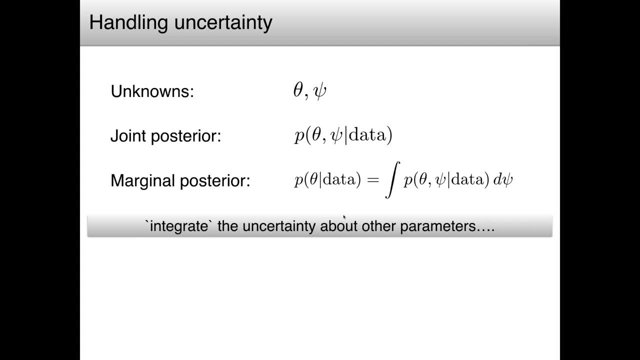 Handling uncertainty. So this is one of the sort of basic features of Bayes that you know that we're always. you know we understand that data doesn't tell us all the information, even if it's big data, It doesn't have for things we're interested about. 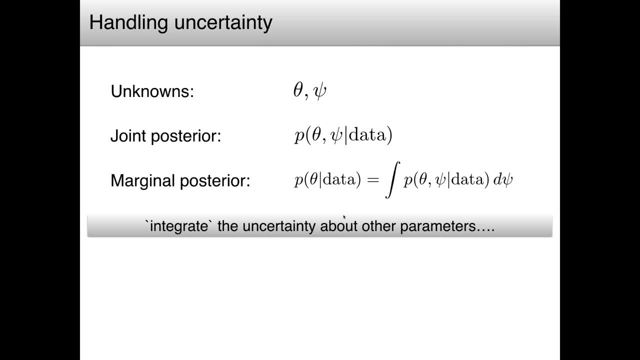 it may not contain all the information, So we have to be able to express our uncertainty about things that we don't quite know, And Bayes is rigged up for that. So let's say, in addition to a parameter, theta, that we might be interested in. 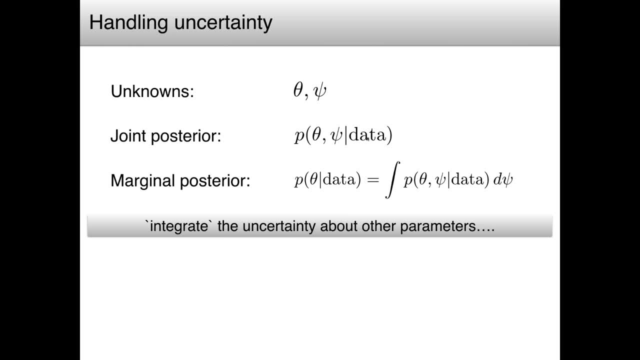 there's some other parameter: psi And Bayes procedure, somehow or other, through a model specification, gives rise to a joint posterior distribution of all the unknowns, given the data that we have. Well, if we're really just interested in theta somehow, then 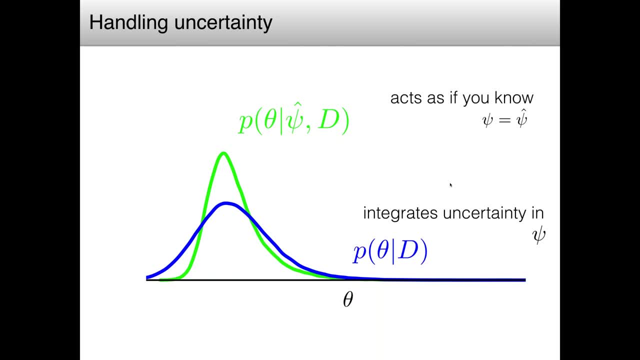 it's going to give rise to some of the other problems that we're interested in. So there's a couple of things that we can consider. I think one thing from a statistical perspective that's really important is that there is a degree of uncertainty. 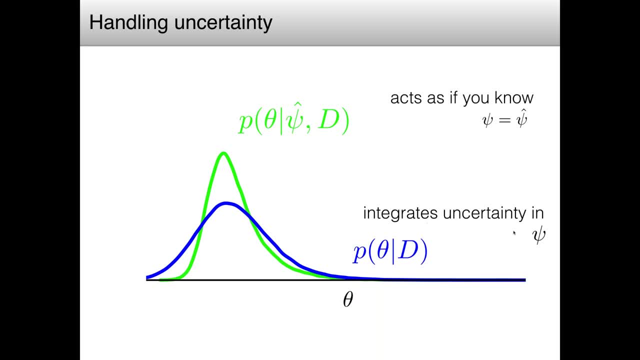 in the way that we're doing our research, And in some cases there's a degree of uncertainty in the way that we're doing our research. So this is something that we can just get back to when we're doing our research And then we just have to think about you know. 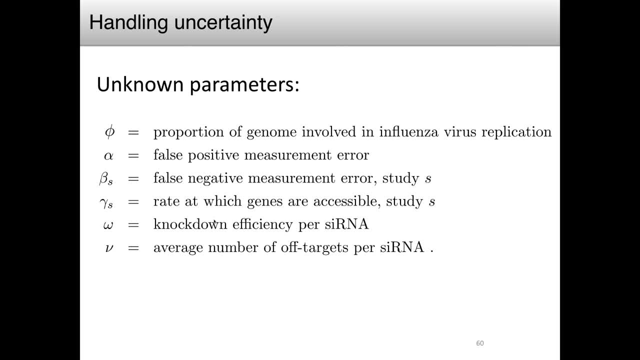 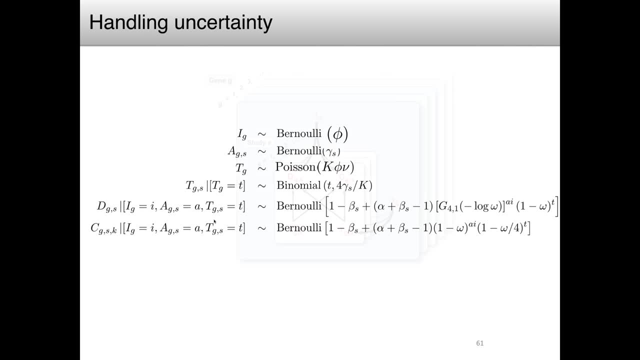 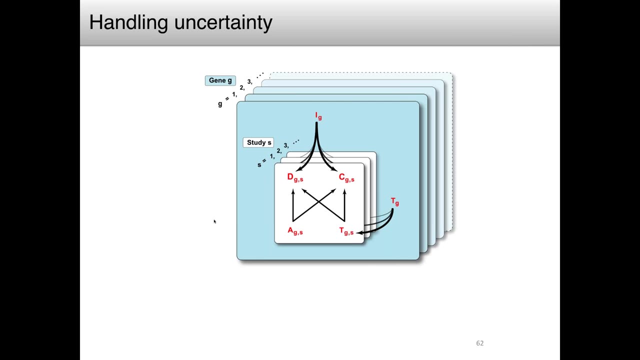 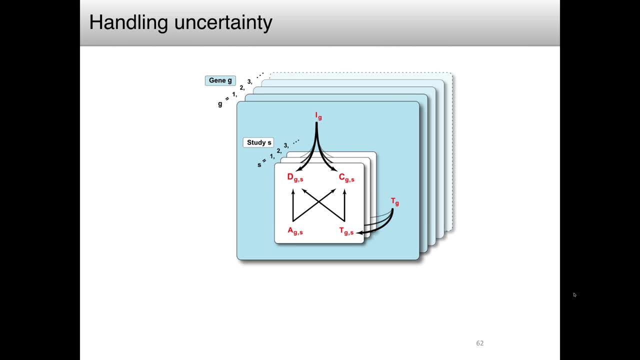 mean, i don't know how far, how long i was. uh, we lost you for actually a few minutes. so, um, maybe you just back up a little bit. that would be good. okay, okay, sorry about that. i don't know quite what happened. let's see if i can back up here. 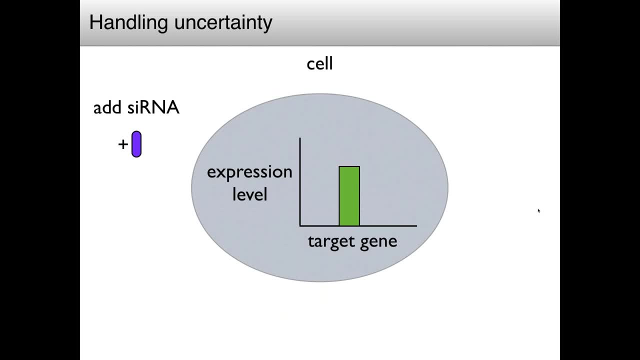 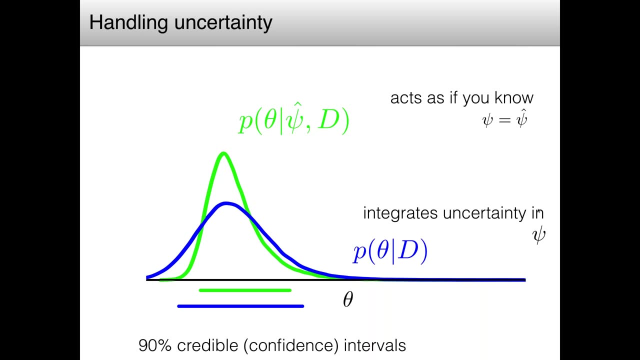 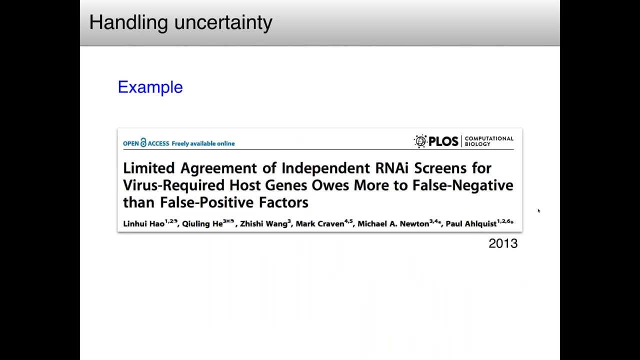 okay, should um? did we give me a sign here? do we know about this part? i think that's good. okay, so the handling uncertainty part i'm going to try and talk about in the context of an example. would that be a good place to kick back in? 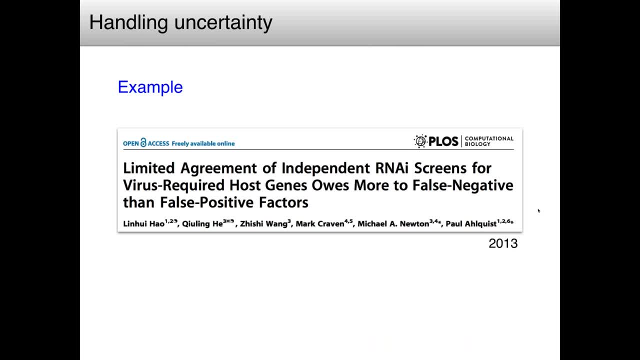 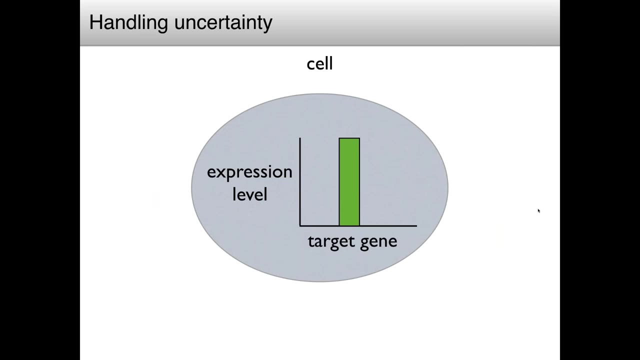 yes, okay, okay, sorry folks. well, um, yeah, so the this handling uncertainty. i'm going to talk about an example, uh, from rna interference. uh, this is a genome-wide uh technology for understanding gene functions and uh, just briefly about that. uh, you've seen the slides but didn't hear me say: 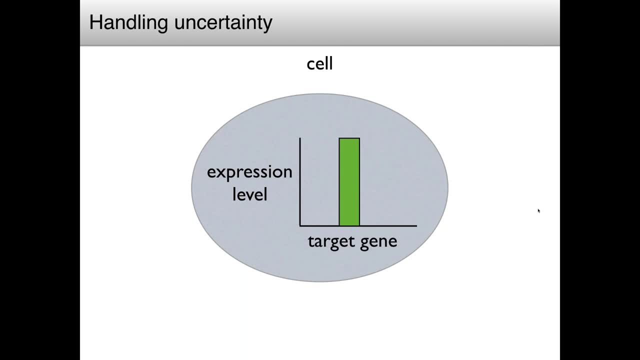 uh, it's a cell-based assay. the basic idea is: you have a target gene that you're targeting with a given si rna. you add that si rna- small interfering rna- to the cells and, uh, what's supposed to do is knock down the expression of that gene. 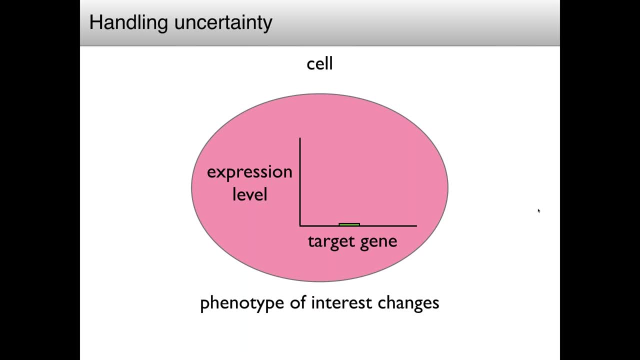 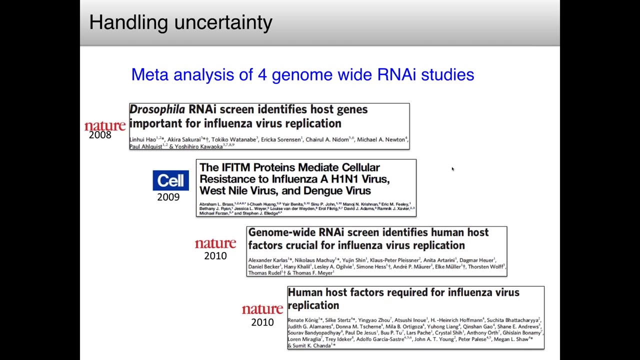 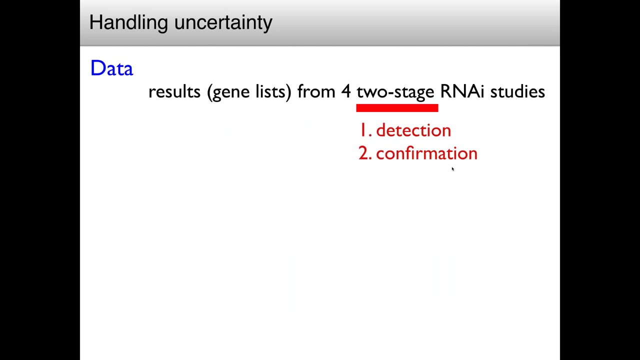 and uh. if that targeted gene is involved in some phenotype that you're measuring, then that phenotype will change and the cell will change as indicated with the red uh. now in and in the story we're talking about, the phenotype has to do with the cell's ability to replicate virus. there are four large-scale studies that use this technology, genome-wide and uh. we had data on on parts of these studies. there are all studies that interesting similarity. they were two-stage studies with the 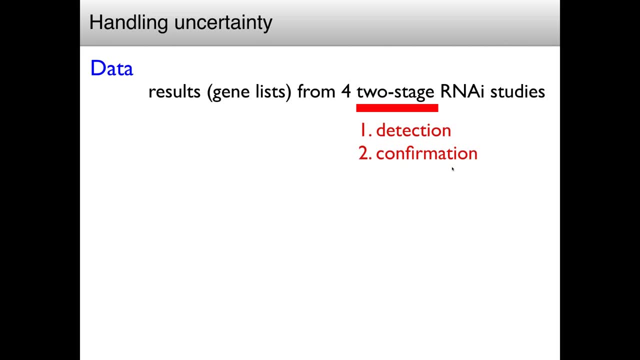 stage studies with a detection screen and a confirmation screen. The whole genome was every one of the genes. different siRNAs were used to try to knock down things and anything that passed the detection screen went into a confirmation screen. that was more intensive but it only had to be applied. 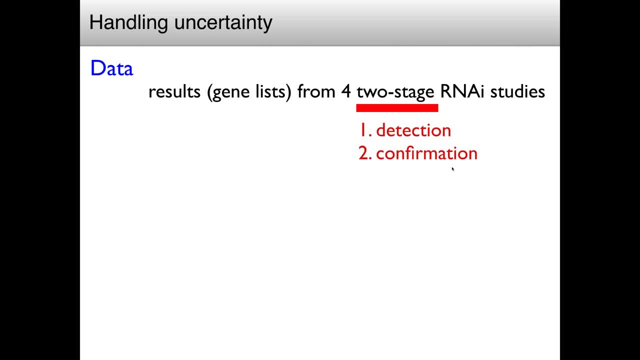 to the things that were detected initially. You remember the detection has to do with whether or not the phenotype here is whether or not a cell, when it's infected with virus and you knock down the gene, whether that changed the cells ability to make virus. One of the curious things here, as in other examples. 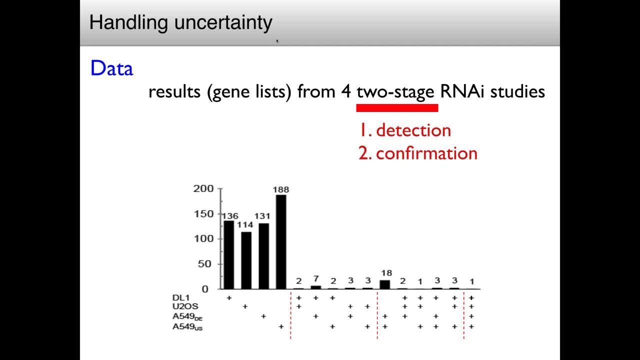 is that, as I was saying, each of the studies made about 200 genes found, about 200 genes that they said when you knock them down it affects the cells ability to replicate virus. but only one gene was found in common to all four studies. A few genes were found in three of the four studies, some in two of the four, but 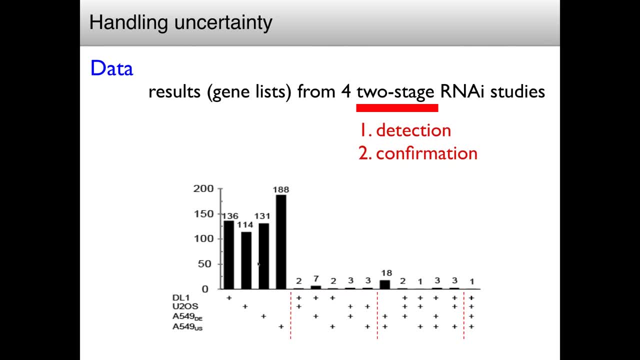 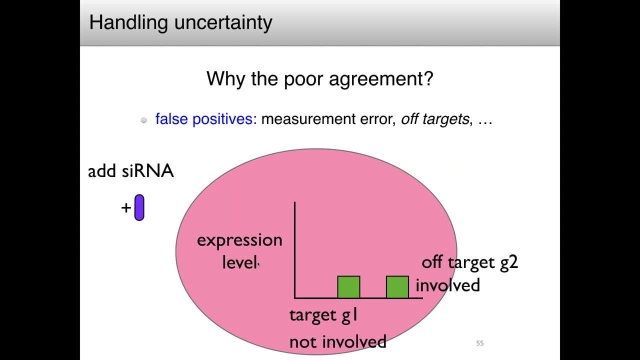 the majority of genes that were identified and reported as involved in flu were uniquely identified in one study only. Could be because of false positives. measurement errors. one but off targets is a big possibility where you add the siRNA and there's a change in the cell as indicated by the pink. but 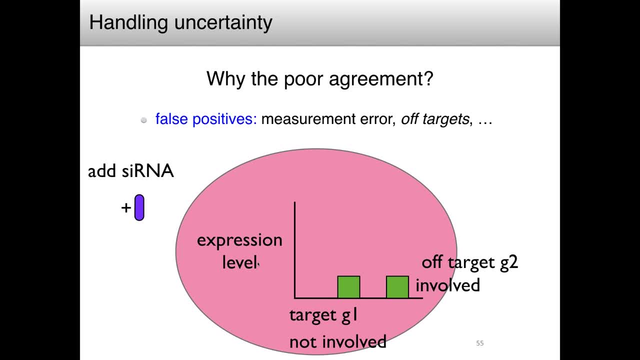 actually the gene that that siRNA is targeted isn't really involved in flu at all. It's just that the siRNA accidentally and not by design- happens to knock down a cell. It's just that you knock down another gene that is involved in flu and then you see the. 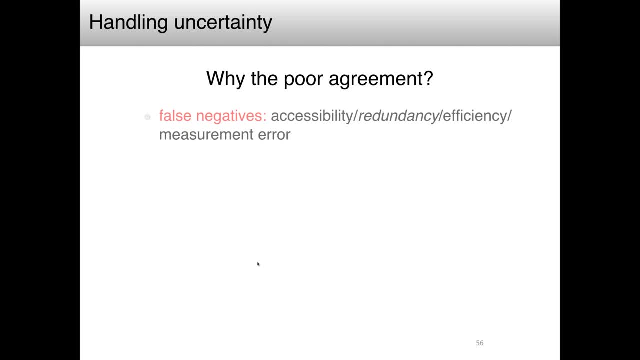 phenotype, even though you shouldn't have. really, It could also be false negatives and there's a bunch of possible false negative results. one possible where it's just the genes really involved in flu but you're somehow not able to see it. when you do the siRNA screen, For instance, you add the siRNA screen, you 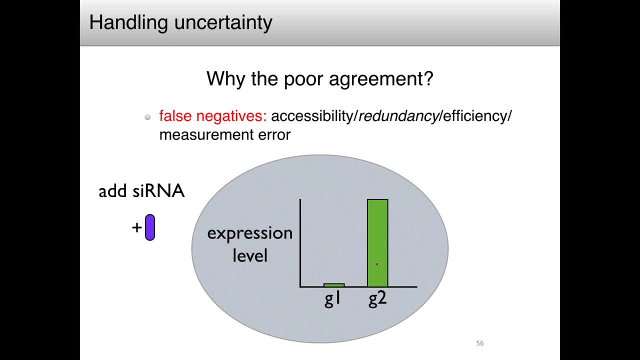 knock down the gene that's really involved in flu, but somehow or other there's another gene sitting there that's doing the job, The first gene in those particular cells. and so, even though the gene one has been knocked down and is really involved, you don't see a phenotypic effect in those. 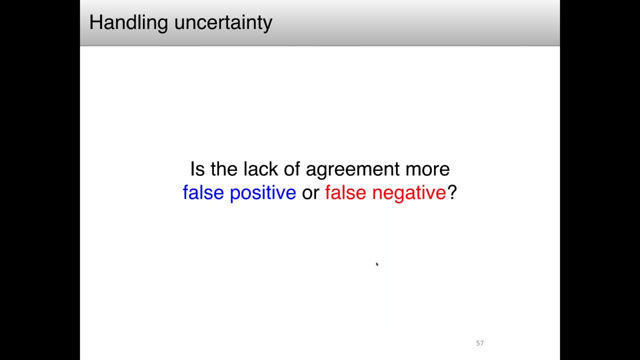 cells. There's a various other forms for the negatives and positives, but the big issue was whether or not it was where which is which is the source of disagreement. If false positives were really a big deal, you wouldn't be surprised to see the lack of agreement, because each study is just pulling them off. 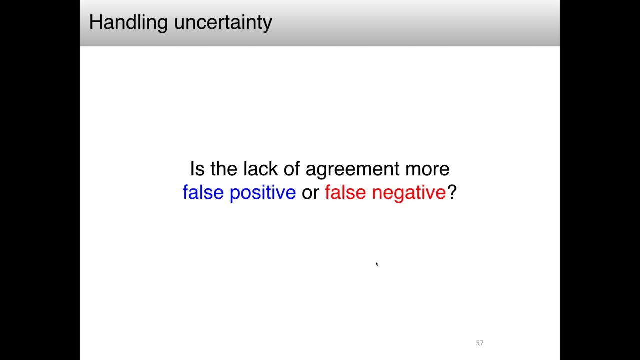 a bunch of random genes, and so it wouldn't be surprising that you wouldn't have much agreement. At the same time, it could be that the flu is really a big, complicated thing and in each of the studies really is just seeing a small part of it, and then the lack of those singletons really are true. 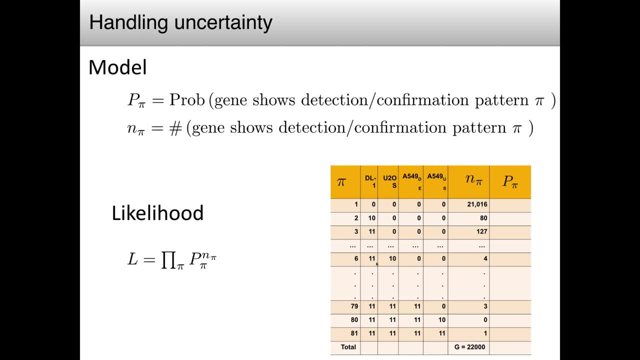 As I was saying here. so to bring it back to the context of Bayesian analysis, we have a probability model for the data we were able to compile, and the data that we're able to compile is a kind of meta analysis of what happens to each gene across each of the studies, whether or not it was. 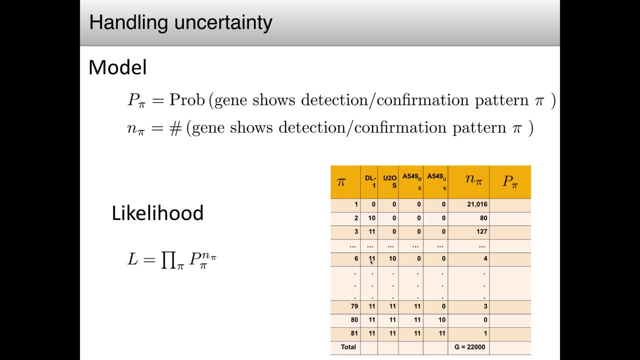 detected and whether or not it was confirmed, and we have counts, for instance, how many genes or four genes that were detected in the first study and confirmed they were detected in the second study, not confirmed and they weren't detected in the second two studies- Naturally a multinomial. 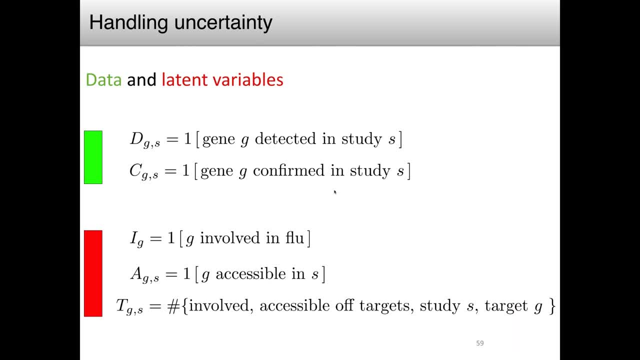 likelihood, and that's the green, is the data that we have- detection and confirmation information, but we don't know a lot of things. we don't know whether the genes really involved in flu. we don't know If it's accessible or if there's redundancies in that case, we don't know. 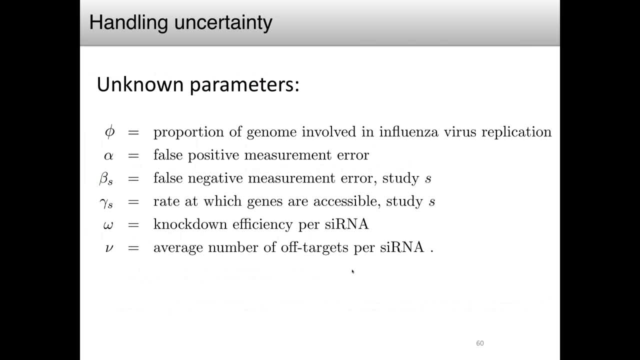 off targets in that study for those SRNAs used and we don't know a bunch of things generally about the system as a whole, about the rates of measurement error and efficiency. We have bits of information about that, but all those things we don't know We can collect, we can put our heads together and try and 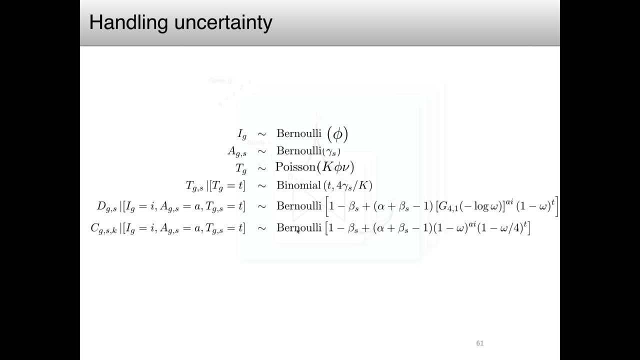 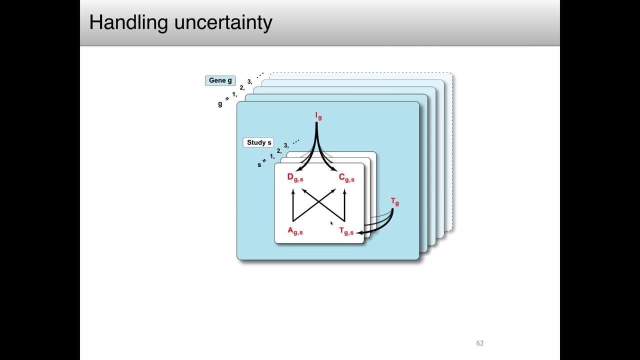 figure out a probability model that links together all those things we don't know with what we know. You often see these, these directed acyclic graphical representations of probability models, to express dependencies, and that's what that is. here We use the tools of Bayesian analysis to come up with a probability distribution of the unknowns. 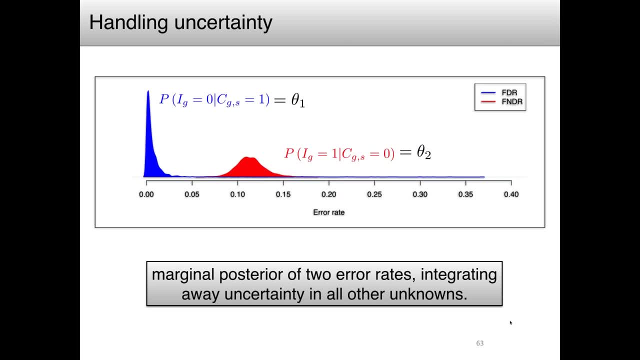 given what we do see, Without going into any of the details of how the calculations go ahead. we work out a joint posterior distribution and then we come down to the statement of marginal posterior distributions on quantities that we're actually directly interested in, these error rates, For example theta. 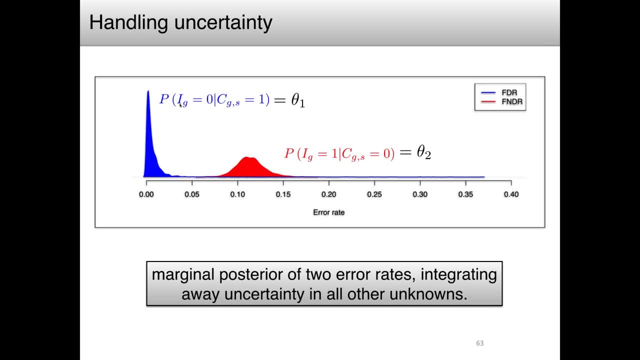 one is a quantity of interest, It's a false discovery rate, It's asking, It's something we don't know in advance. really, It's the chance that the gene would really be involved in flu, if in fact it was confirmed in the study. 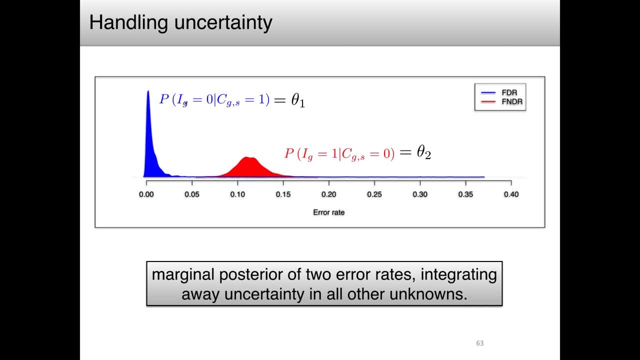 Pardon me, let me say this again: It's the chance that the gene is not involved in flu and that's the IG zero, given that it's confirmed. So if it's confirmed, that's the chance it's not involved. That's a false discovery rate. This is a kind of a 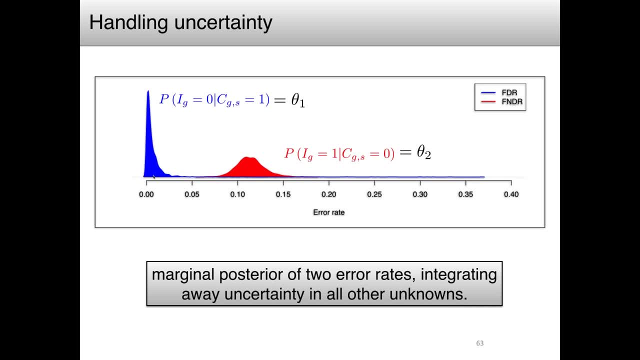 false positive rate. Well, we don't know that false positive rate, but in our calculation we get a posterior distribution. We get a distribution for the false positive rate That's way down here, and similarly we get a distribution for the false negative rate And this and some. 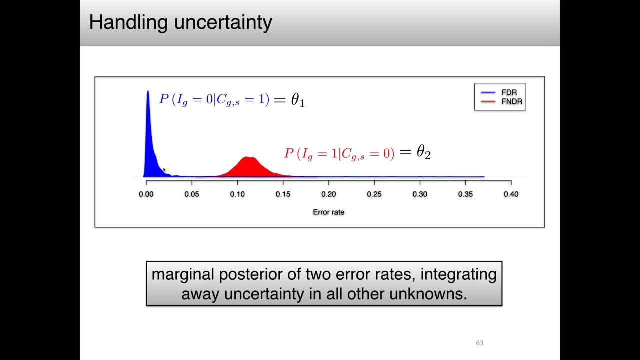 other similar calculations. basically, they've accounted for all the uncertainty and all those many, many things we didn't know in the context of a specific probability specification, And it tells us pretty unequivocally that false negatives are a bigger problem than false positives, And that lines up with 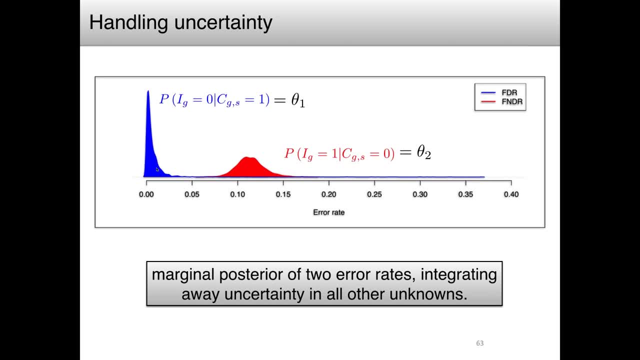 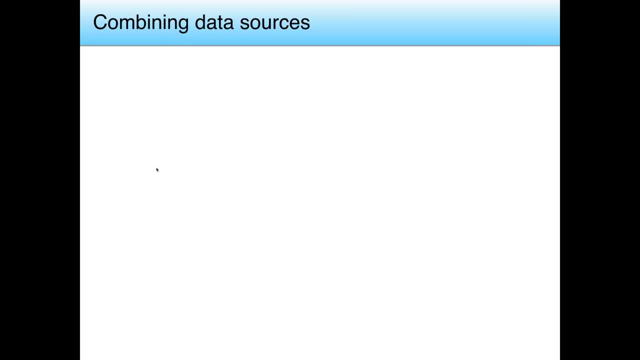 some other other analyses of the same data, But that's an example of using marginal posteriors to get at particular quantities of interest and address those. Ok, I'm going to move on to another example, Combining data. This is where, so one 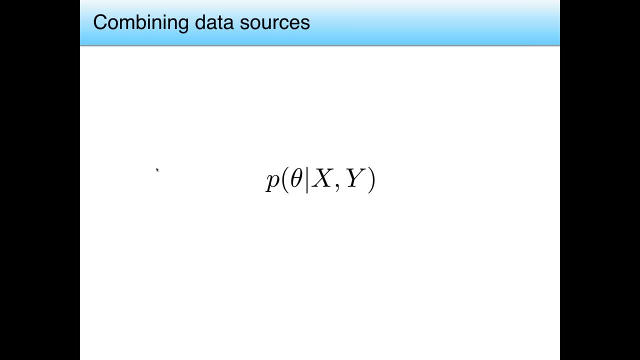 of the big things about Bayes is that you can combine multiple data sources, So I'm going to talk about different data, X and Y, coming together to make inference. This is a story about cancer and it's based on this amazing, crude creature called an aggregation chimera that is formed from two early embryos that are 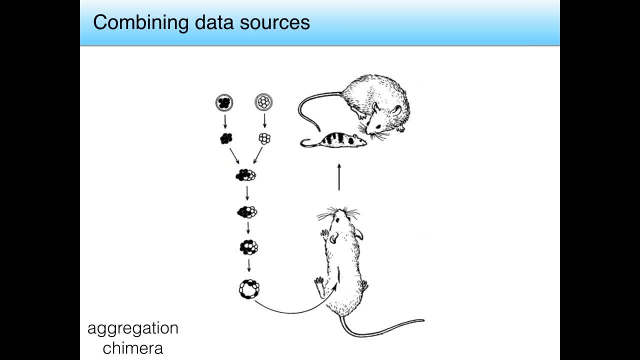 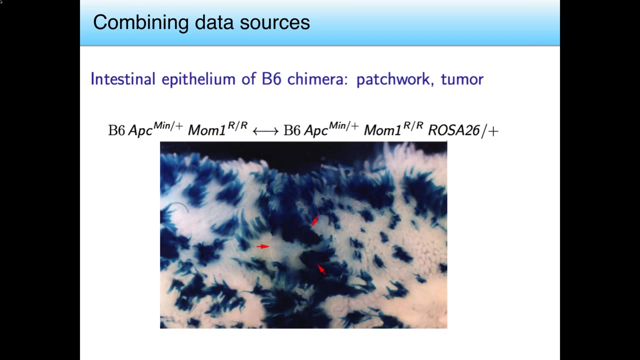 fused together and planted into a foster mother and then, once in a while, if it all works right, you get some animal out. That's really two separate animals, more or less merged together for parents. Here's a chunk of an intestinal epithelium of one of these animals. It's also been genetically engineered to be. 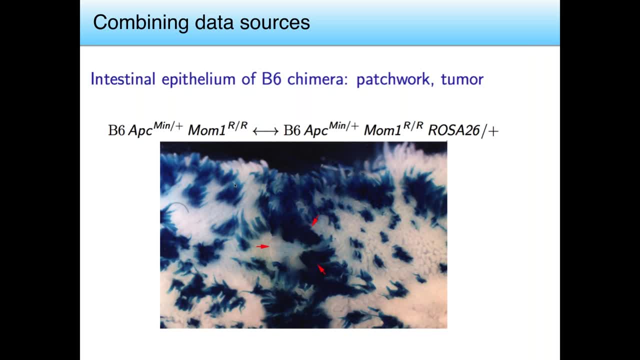 susceptible to cancer. So this is an example of an aggregation chimera that's very susceptible to growing tumors in their intestine, and it's blue and white color owing to the two separate parental lineages. This is, the blues come from one side and the whites come from another. Now, curiously, in the 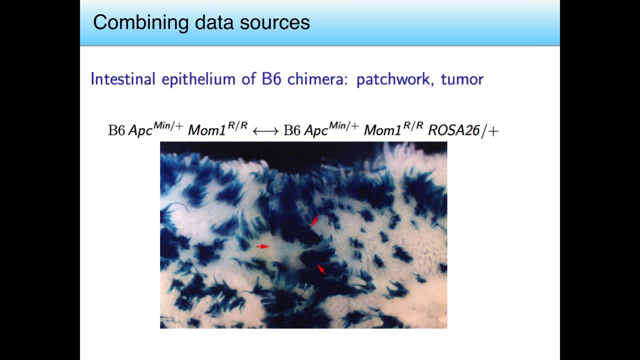 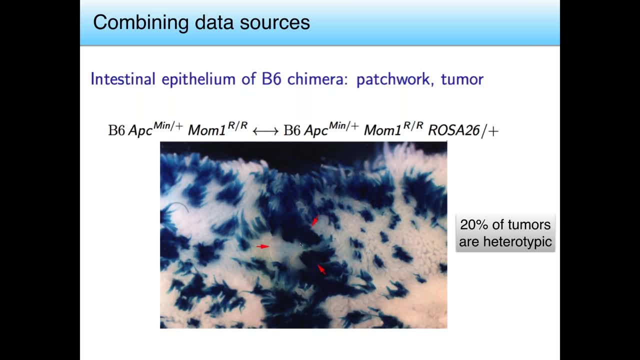 But the standard story about biology and cancer growth, which of course, we can't. well, that's one of the cool things about cancer research is that we and statistics for cancer research is you're talking about events that happen before you're able to observe them, But the standard story about tumors growing out. 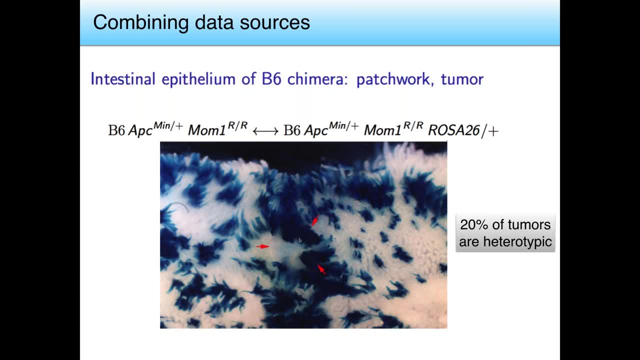 of crypts. crypts being clonal doesn't work here, because if it did, they would be either pure white, as the cells in one lineage come are either white or pure blue, but they wouldn't be mixed together. So this is like a. this is a kind of a polyclonality story. Now there's a bunch of interesting. 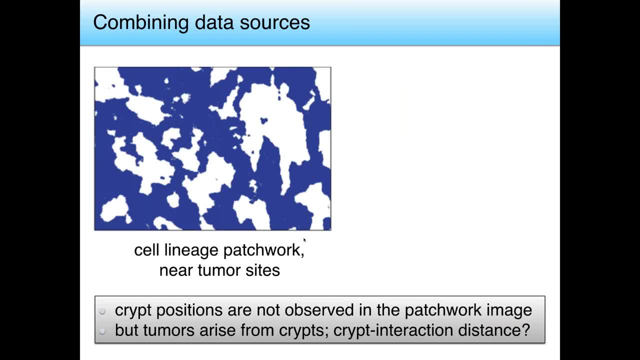 statistical issues with the polyclonality. I just want to focus on one specific one about combining information sources. So one information source is to do with the patchwork of the cell tissue of this lineage. Some of the cells come from one lineage, one of the originating embryos. 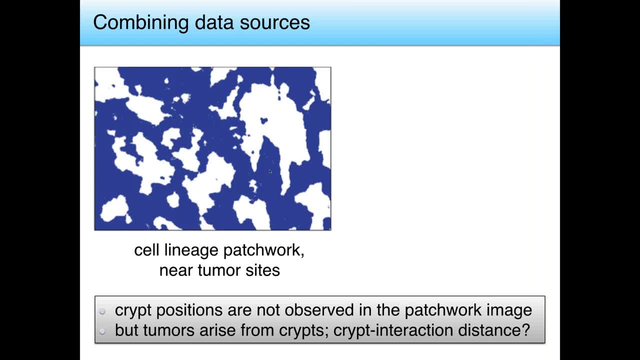 some come from the other. So that patchwork, the beautiful patchwork that presents itself Now, we'd like to know, in order to have an understanding of tumor initiation events. we'd like to know where the crypts are under there, but we don't get to see those. Now, on the other hand, that's something that well. 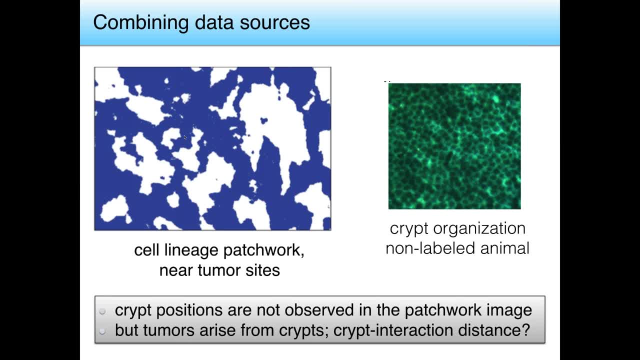 just to back up, There's something about the imaging technique that it's not able to reveal the positions of the crypts and the blue white images. Now there's data on other animals that aren't animals, that are chimeric animals, but their data on other animals, or at least they're not blue white image. 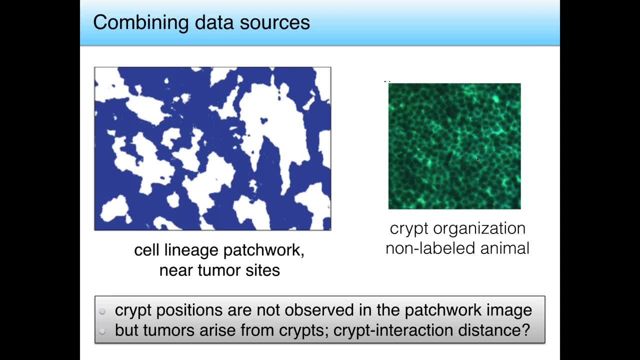 animals. So we can see that it's a very mother. So you know we've got two different populations here. Some семьes are white, some are blue white, some are blue white. that show what these crypts organization look like. 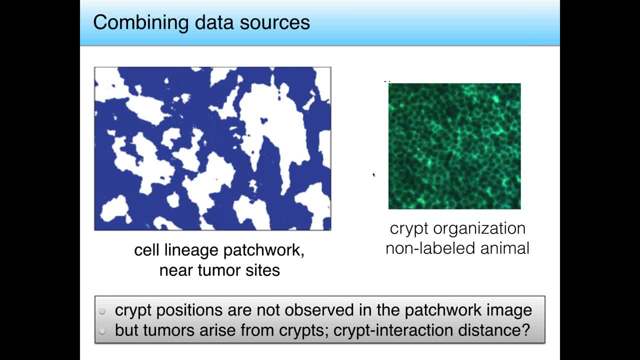 So we'd like to kind of merge, fuse this data with this data somehow, And that's what the analysis that I'll show tries to do. The reason we want to do this is because we're trying to understand how many pairs of crypts 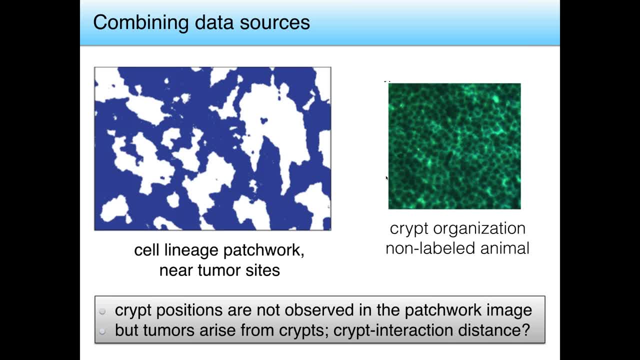 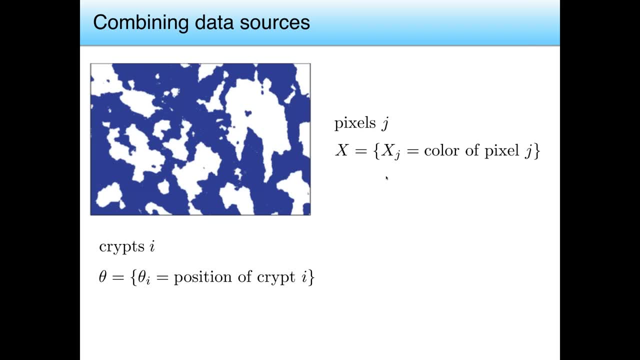 are really on edges between blue and white that could potentially give rise to these polyclonal tumors. So the data on one side, the x, is a pixel image, a blue-white image, The unknown quantity, theta, are the positions that we record as centers of positions of. 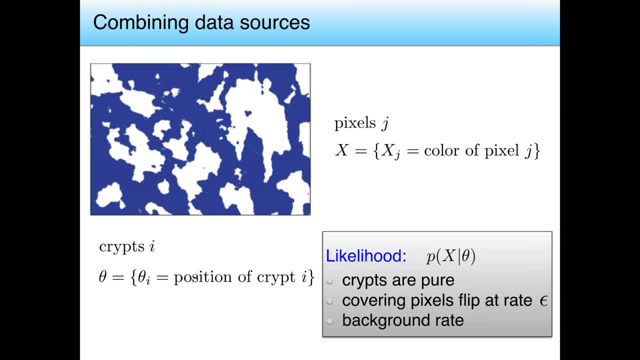 crypts And it's easy, with some simple image analysis ideas, to work out a likelihood. If you knew where the crypts were, what's the probability of seeing a particular image? You know that the crypts are pure blue or white. There would be some flip error at some small rate which would flip a pixel. 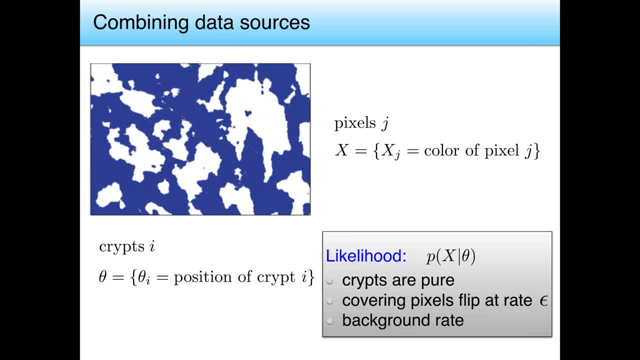 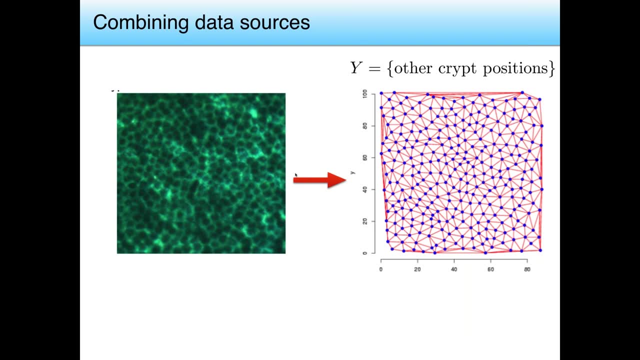 If it's supposed to be white, it might be blue, And then if you're a pixel that's not over a crypt, you might be coming up by a background rate. So that's one part. Now we also have a second data source. I was saying about the positions of crypts, not 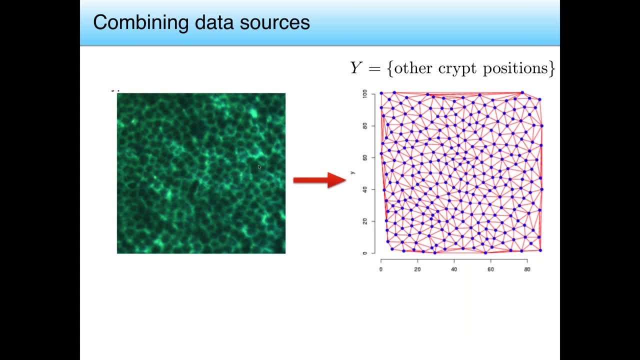 in the data that we're interested in, the blue-white image, but in another source. We can triangulate that image and look at those points. They're not scattered uniformly, randomly around. In fact they have quite a bit of spatial structure that we can express with a kind 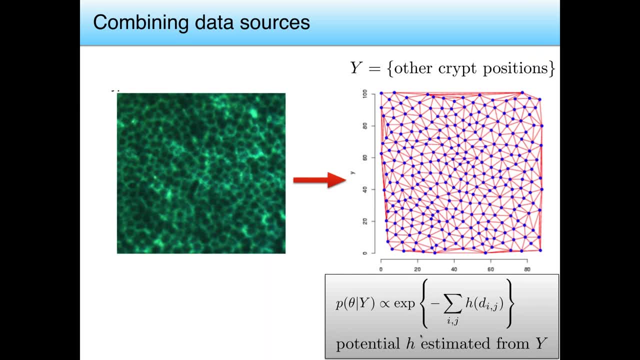 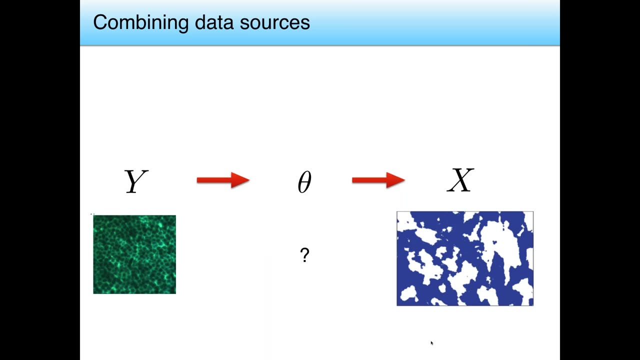 of a spatial analysis. It's a spatial model on positions where we use the actual interpoint distances to get an estimate of this potential function for the joint distribution of spatial positions. So we try and put that together. We use the external data y to tell us about what kind of patterns we might expect to see. 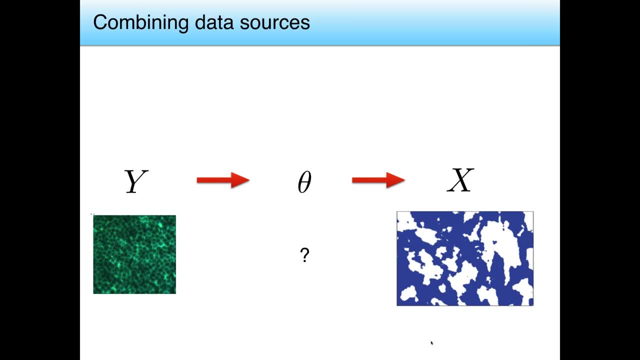 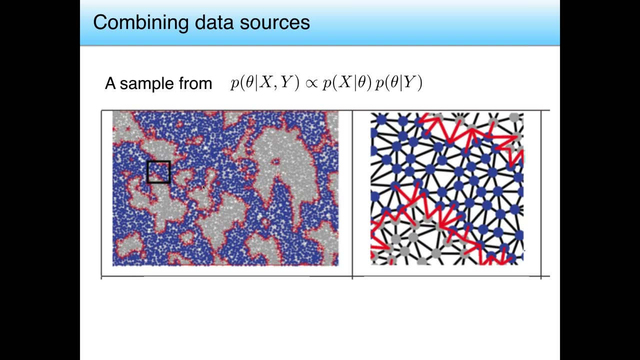 in the crypt orientation theta, And we want to use that to get. we take the blue-white image together to try and figure out what the crypt position might have been. in fact, This is one sample from the posterior distribution of the crypt position that I blow up here. 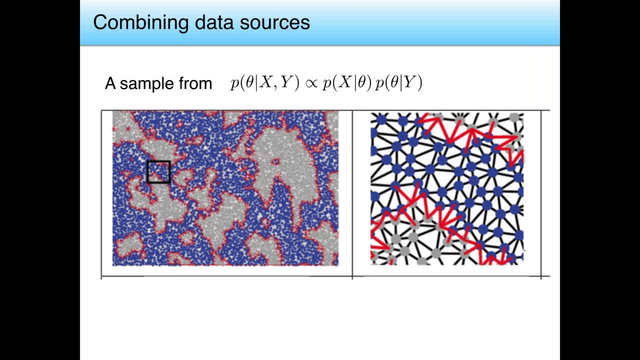 And I've colored the crypts either blue or white, depending on the majority color of the pixels above them, And the key thing had to do with these red edges. These are neighboring crypts that are of opposite color, So if a tumor might emerge from crypts nearby like that, there would be a certain rate at 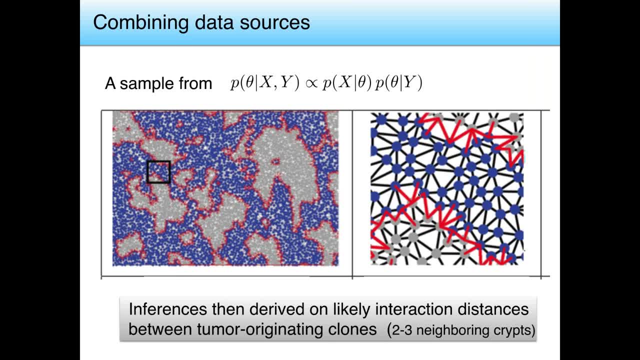 which that happens, that we can estimate, And then so, based on this, we could get some idea of opposite color, So we can get some idea of what the interaction distance might be in between crypts that are at the origin of polyclonal tumors. 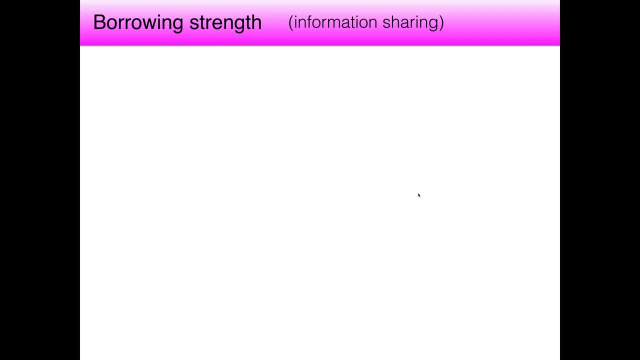 OK, That's a quick run through of combining information And then the last part. I want to, in the last few minutes, talk about borrowing information, borrowing strength on information sharing. This is a big deal. in genomics. You've got possibly many different but related inference problems. 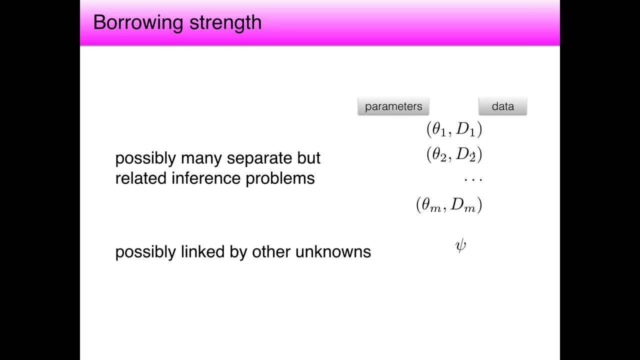 There are M of them And I've got theta. These are the unknown parameters in each one, And each one gives rise to a data set. They're separate but related in some sense. Now there's two cases. The problems may be linked by some other parameter: psi. 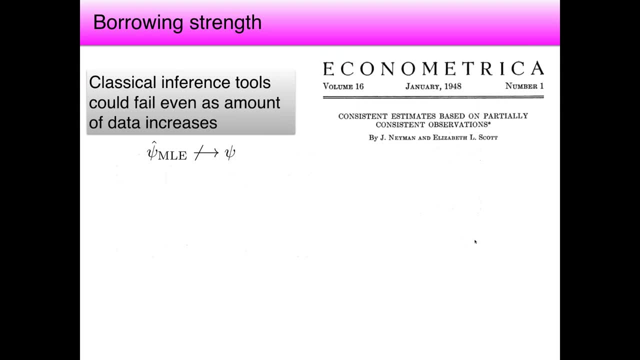 We don't know any of the thetas or the psi's. We get the data Now. it's a classic result going a long time ago that if you're interested in inference about the psi, that unknown linking parameter, you could screw up. 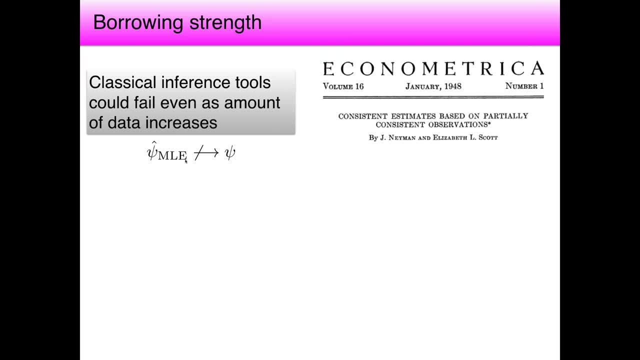 Even if you get lots and lots of data, your standard estimates, the so-called maximum likelihood estimate, It won't be consistent for that underlying parameter. It goes back to Neiman and Scott in 1948.. Just a few years later, though, Kiefer and Wolfowitz showed you could do a trick. 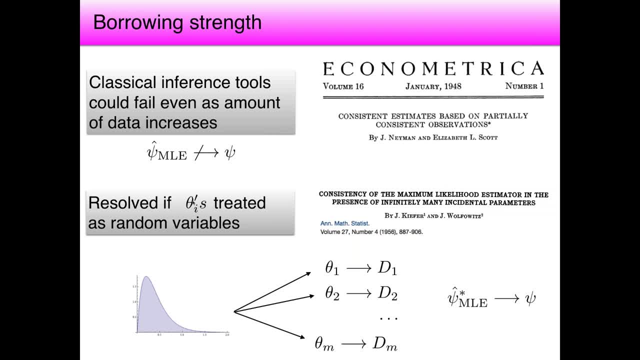 You've got a lot of those theta parameters And instead of just treating them as unknown quantities, you treated them as unknown quantities that came from a distribution And you accounted for the fact that there was such a distribution. Even if you didn't know it, you could get an estimate. 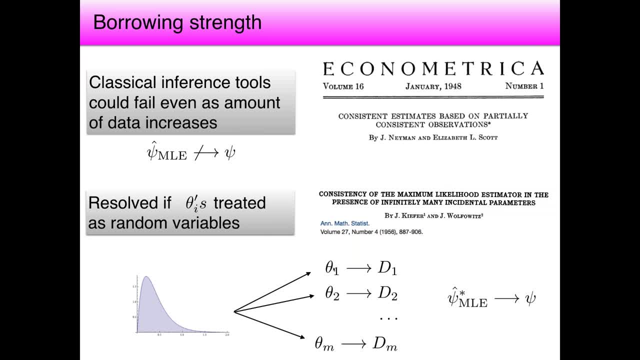 You could get an estimate that now is still an MLE, a maximum likelihood estimate, But it's acknowledging that the thetas are coming from a distribution or essentially random effects, And you could get consistent estimates of the unknown. So there was something just about having lots of parameters. 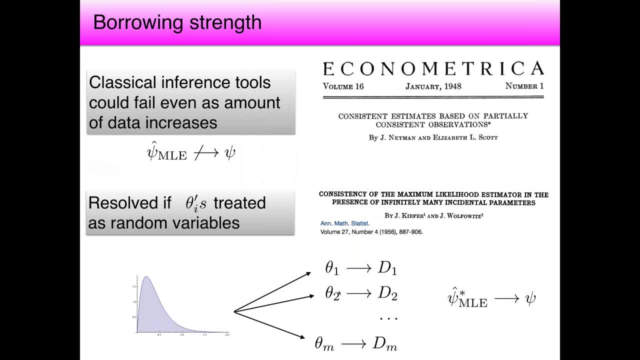 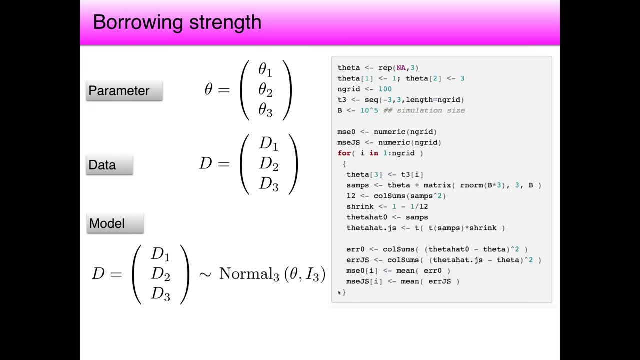 When you had them, you ought to treat them as if they were from a population That turned out to be important. Now here's another related thing that happened long ago too. Here's a parameter. I'll tell the story in three dimensions. 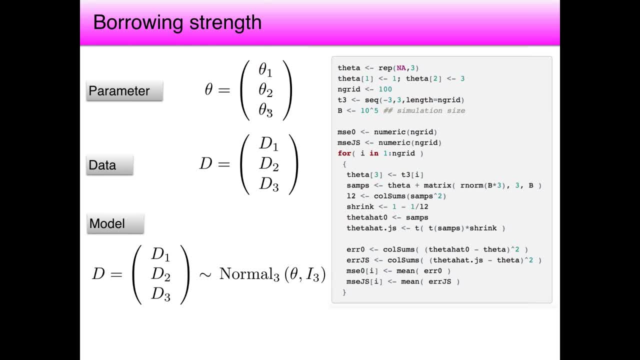 There's three unknown related Separate problems: The three unknown quantities, theta1, theta2, theta3.. And I'm going to get three data points: d1, d2, d2, d3.. And the sampling model is that the data are independent, centered on theta. 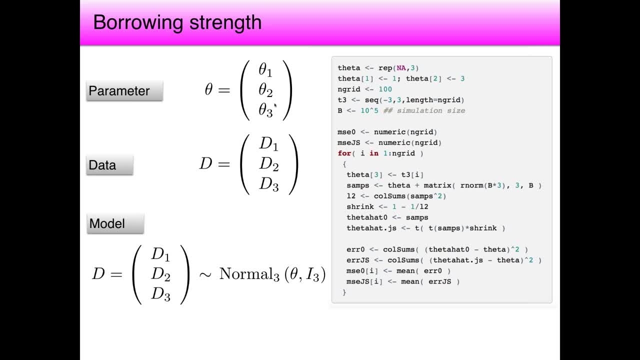 So d1 is a data measurement that's estimating theta1,, d2 is estimating theta2, d3 is estimating theta3.. They're independent things. So d1 has no effect on d2 and so on. The little code chunk on the right is actually trying to simulate that. 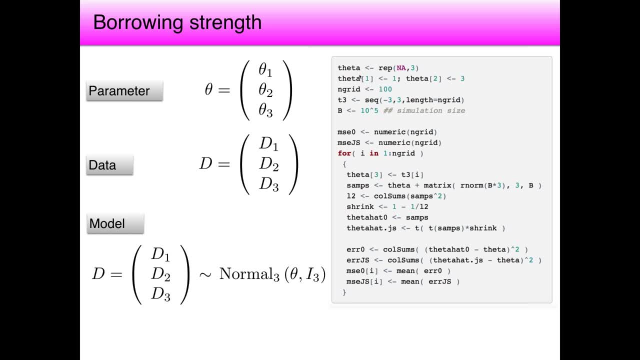 It simulates this for a couple. It simulates this for various thetas. In fact, in this little code, I want to fix theta1,, fix theta2, and I'm going to run on a grid of theta3 to show a picture. 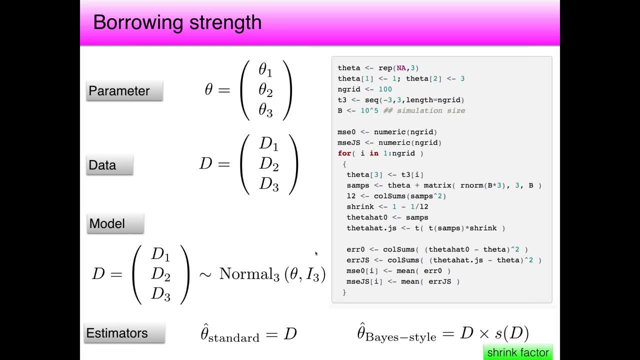 I simulate up some data. Now the question is if I use the data. I want to use the data somehow to estimate the unknown quantities, the thetas. There's no psi in this story, There's just unknown thetas. I could use the standard estimate, which is to use the data themselves as estimates of. 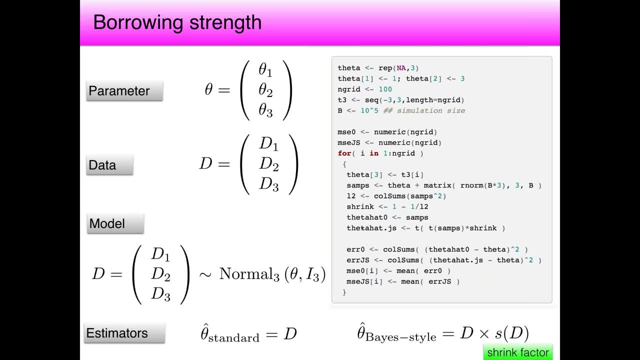 their expected values. That's the standard estimate which I calculate in this code and I look at error of that estimate In a way. I'll show in a second. And then there's another one, a Bayes-style estimate. I'll call it just Bayes-style. 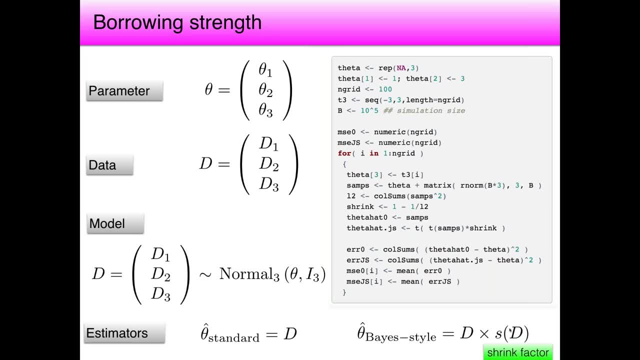 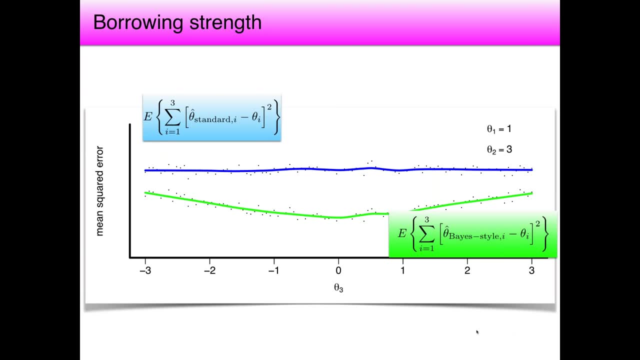 It's the data, but I shrink it a little bit, just like back in this tack problem where there was that shrinkage. There's a little shrinkage here. that is a factor that in fact, depends on the data. Now this is the plot of the error. 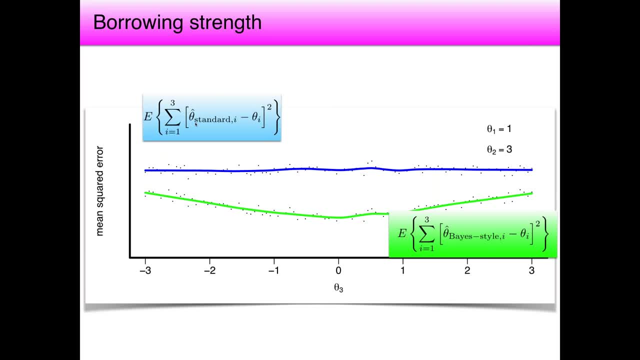 The problems. that were the separate but related problems. They had nothing to do with each other. The noise had nothing to do with it, But I'm going to assess the error of an estimator by combining the problems together and look at the average squared difference between an estimator and the thing it's estimating. 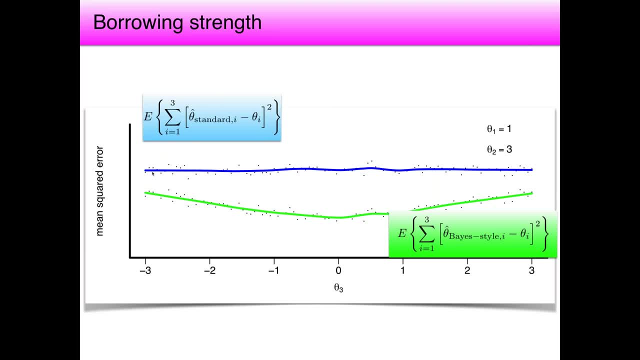 accumulated up over the three different problems. If I look at the standard estimator, that mean squared error is in the blue here. according to that simulation, I'm fixing theta 1, theta 2, and I'm just letting theta 3 vary just because it's hard. 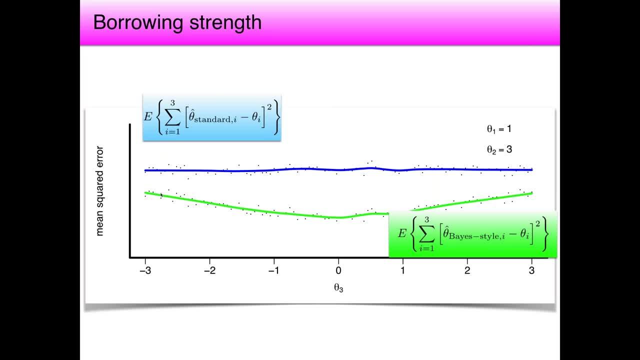 to draw in three dimensions. If, instead, I was looking at the error not of the standard estimator, but the error here of the Bayes estimator, I get a Bayes-style estimator, I'll call it. You get a uniformly smaller, uniformly smaller. 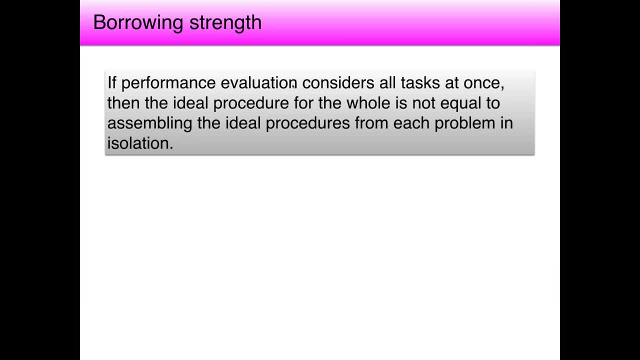 So this is a fundamental finding from way back, that if performance evaluation considers all the tasks at once, all those related but separate problems, then the ideal procedure for the whole thing is not taken by assembling the ideal procedures for each problem to take in isolation. 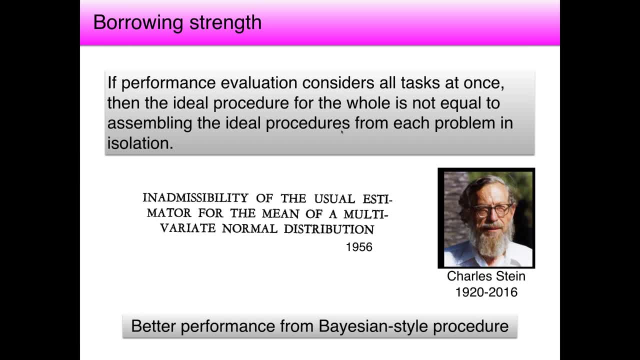 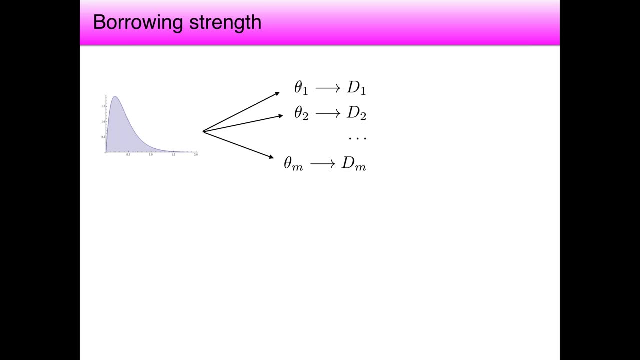 A fundamental fact that Sam Stein figured out and that, in fact, you can actually do better in frequency terms by using some kind of a Bayesian-style procedure. OK, How does this actually work? Well, go back to the Kiefer-Wolfowitz story. 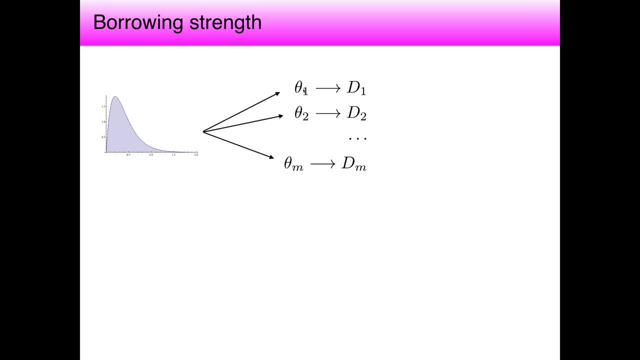 You've got a bunch of related but separate problems of unknown quantities, data, and I'm going to now treat them as if they come from a distribution in order to try and get some benefit. But of course, in reality I don't know that. I know the data, but I wouldn't know the distribution. 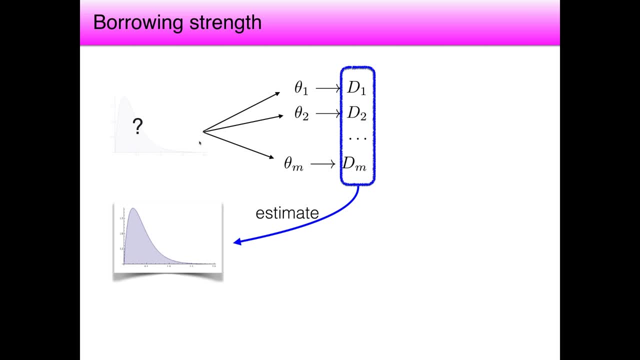 that generated them. Of course I have data, so maybe I could somehow or other estimate that distribution. Now, as I've estimated it, now I can think like a Bayesian and say: well, I have that distribution called g which is essentially like, informally, a prior distribution before. 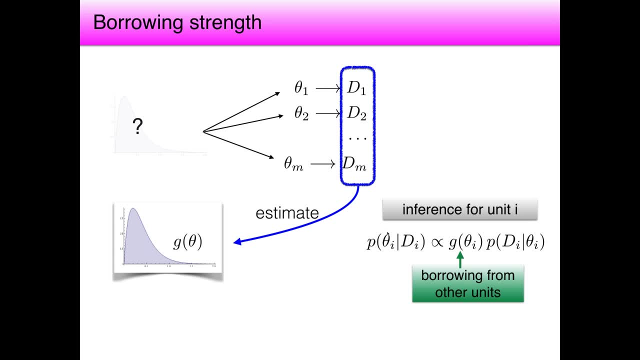 I get data essentially associated with all the parameters, So I can do a Bayesian-style calculation By working out the posterior proportional to that prior times the likelihood piece, And here this is the borrowing information part. This actually I'm doing inference on a single unit, but this has acquired information from. 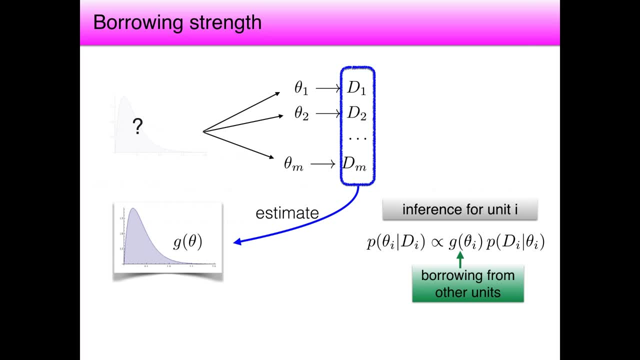 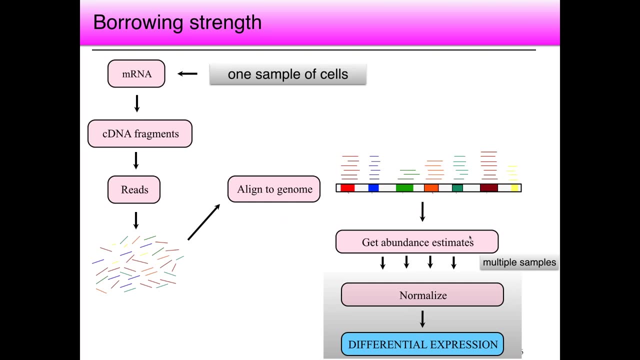 all the other units in this two-stage process. OK, So borrowing information is used a lot in genomics. I'm just going to close out with an example: RNA-seq, which is used for measuring transcripts. quickly We get samples of cells. Their RNAs are extracted. they're converted to cDNA. they're read by next-gen sequencing reads. Those reads are aligned to the genome. We get some rough raw measurements of how frequent those RNAs are in the sample of cells. We have to do some computation to get abundance estimates. 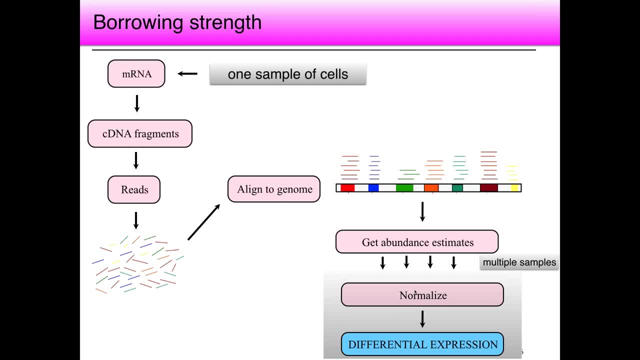 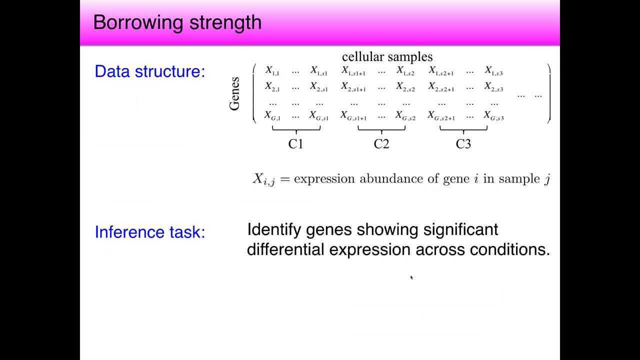 You'll get multiple samples together, You'll normalize them to account for sampling specific artifacts And then we get down here to a problem of differential expression. We want to know which genes Which genes are significantly differentially expressed across different conditions And the basic data structure that comes into the calculation. we've got genes on the rows. 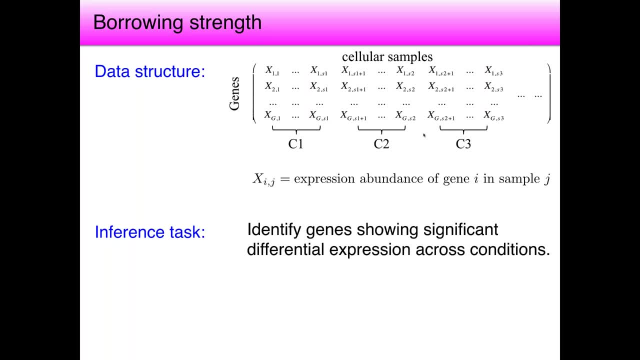 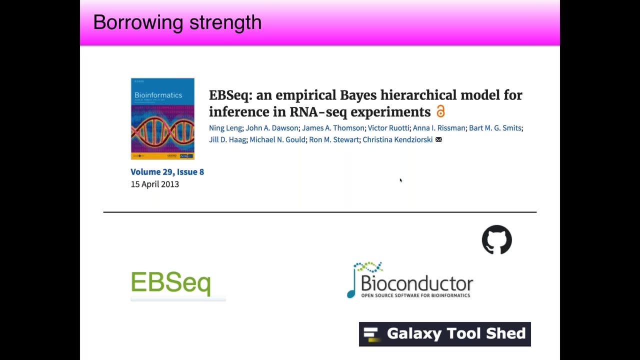 We've got different samples along here And those samples can be bundled up into multiple conditions. The basic measurement after all that processing is some measure of expression, abundance of a gene i in a sample. I'm going to just say briefly something about a popular technique called EBC which is deploying 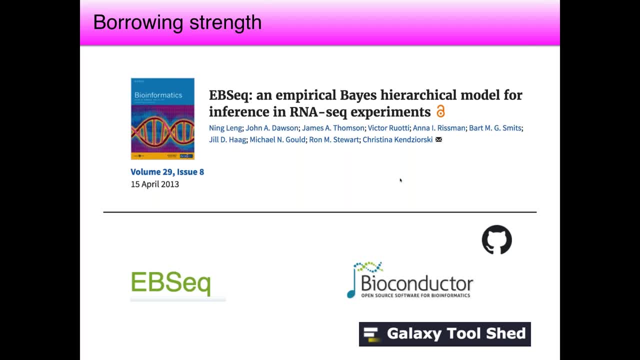 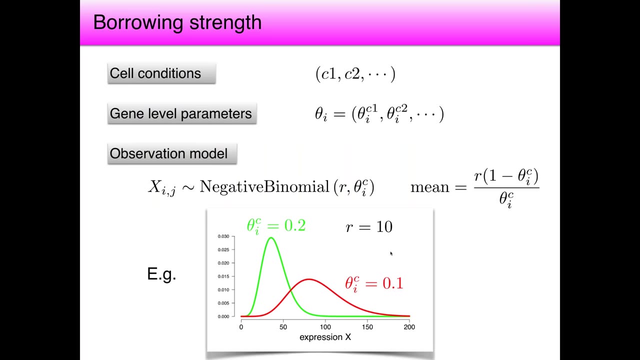 one of these information Sharing tools in the context of expression, And it's a popular one because it has some nice statistical properties. You can get it at those places. Let me say quickly: I've at my 1150, but I'm just going to just finish up with a couple. 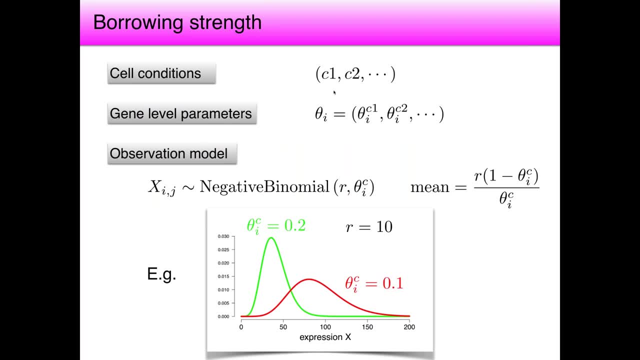 of slides on the structure of this, if that's OK, Alex. Yes, it is, Keep going, Thanks, OK. So how does the structure of this thing go? You've got multiple cell conditions. You've got gene level parameters. 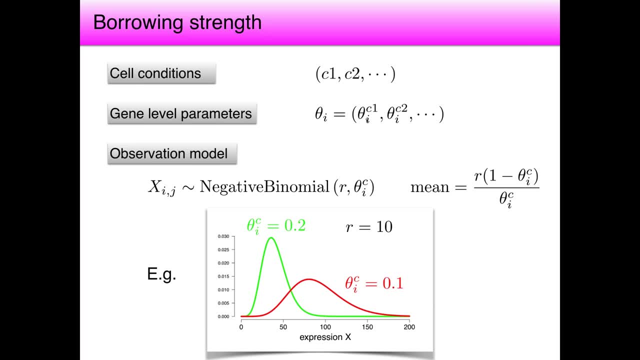 So these are parameters that have something to do with the distribution of the expression measurements. in each condition You get replicated expression profiles in various conditions 1,, conditions 2, and so on, And each gene i is going to have some property. So, for example, if we took the negative binomial distribution, which is an over-dispersed 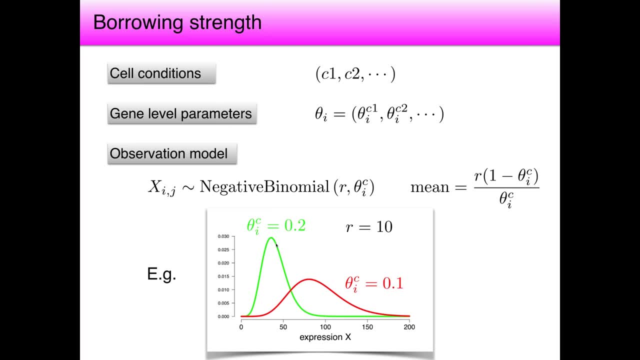 a natural distribution to use for count data. I show for two different thetas here, possibly two different conditions on a given gene, what the sampling distribution of the counts might be like for different expression values here. If theta c was, if 0.1 was the expression, then if theta of 0.1 was the value, then this: 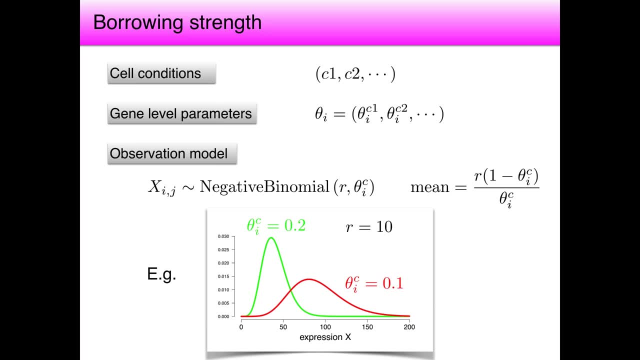 would be the fluctuation we'd expect to see of expression measurements in that condition. So at issue. so this is a natural probability distribution used. many people use it. But how can you use it in a way to borrow strength? At issue are: 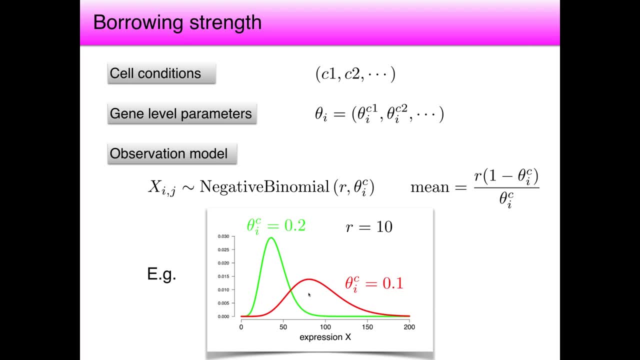 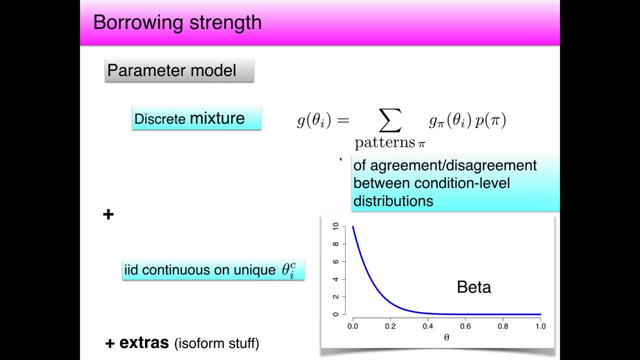 At issue are, you know, you want to find genes where there may be really some difference in the thetas between conditions. So, coming to the borrowing strength part, we have a bunch of related but separate problems, those being the related, all the different genes. 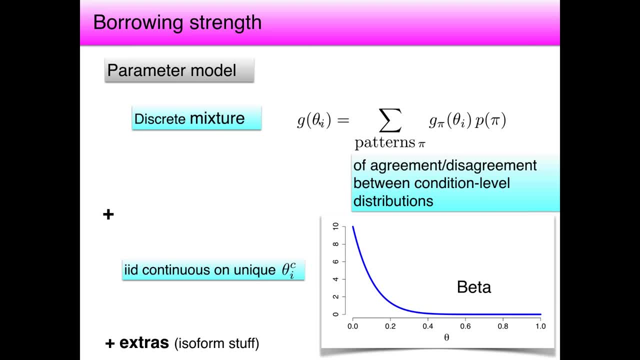 And we have parameters, theta on one for each gene and each one is a vector over the different conditions. And the key structure of EBC is to do a first discrete mixing over so-called patterns of agreement and disagreement between the condition level distributions. 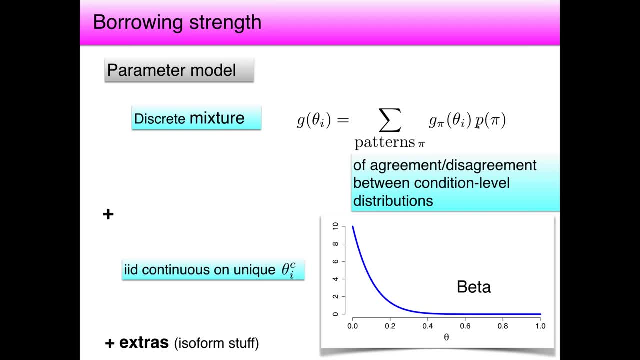 And then for any latent variables. so that's a finite sum here. I'll give a quick example of that subsequently. And then you'll still have unknown thetas, even if you. even for a given pattern you'll have unknown thetas And they'll come out of some mixing distribution as well. 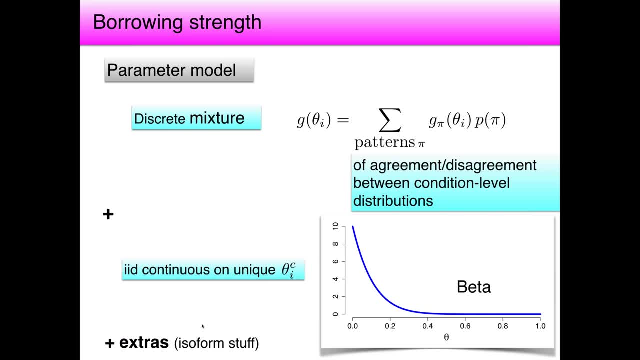 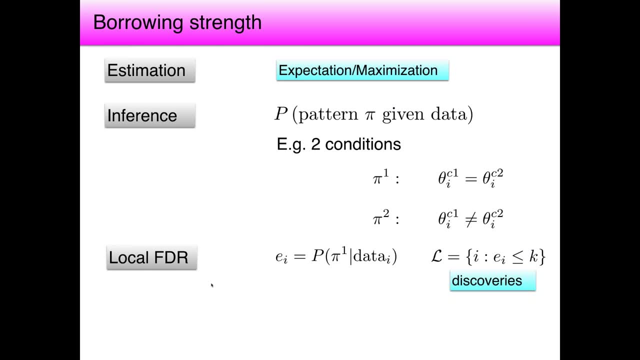 EBC also has some extra bells and whistles that handle isoforms nicely and some other things that I won't say anything about. So that's a specific structural model for that distribution gene. We want to learn that from the data, so we use the M algorithm to do it. 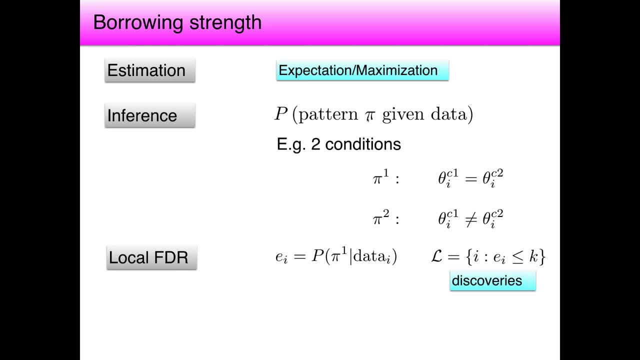 Once we've learned it, we can apply Bayesian-style calculation. What's the probability of a given pattern, given data? And here's where the patterns come in. For instance, one pattern if you have two conditions. one pattern is that the thetas. 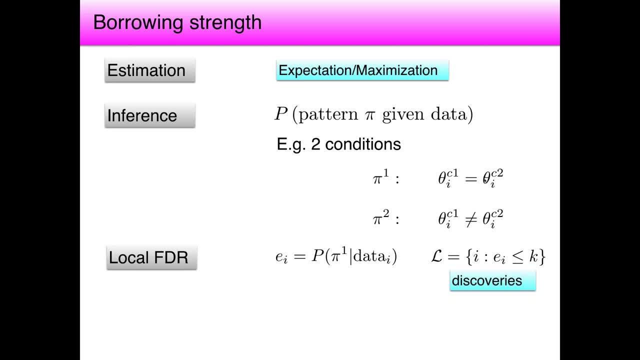 on that gene, for the two conditions are the same. This is the no differential expression: that there's no real difference between the two conditions in the average expression of the gene, Or another pattern might be. there really is a difference in expression on the average. 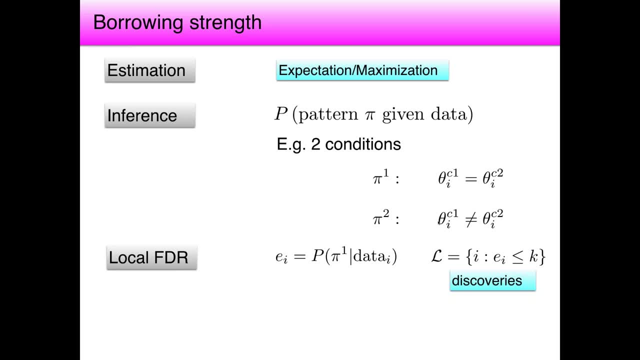 between those two conditions in the expression of that gene: Basic, null hypothesis, alternative hypothesis at the gene level. But the key thing about EBSIG is it's leveraging all the information across the genome to try and improve sensitivity and improve statistical properties of the final procedure. 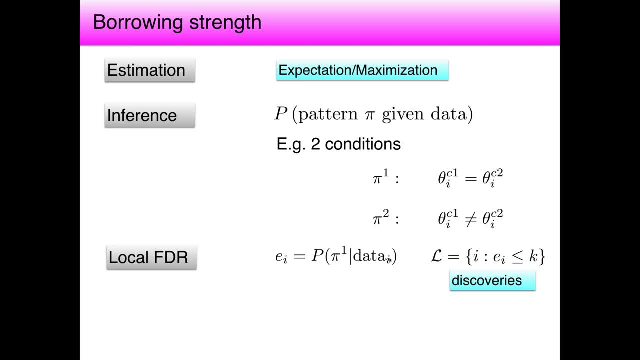 And part of that are local, so-called local FDRs. probability of the null being true, given the data And the list of discovered genes, would be the things where that null probability is small. And then if it's null small, then there's a high probability of the alternative. 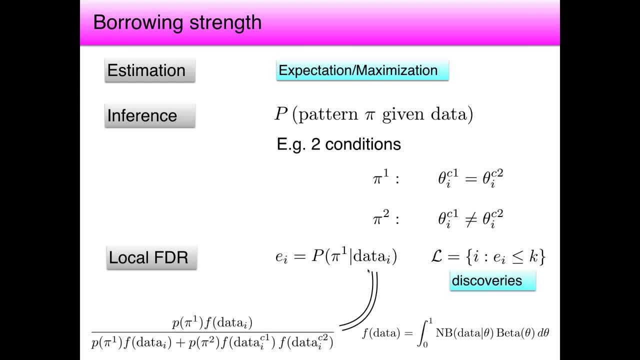 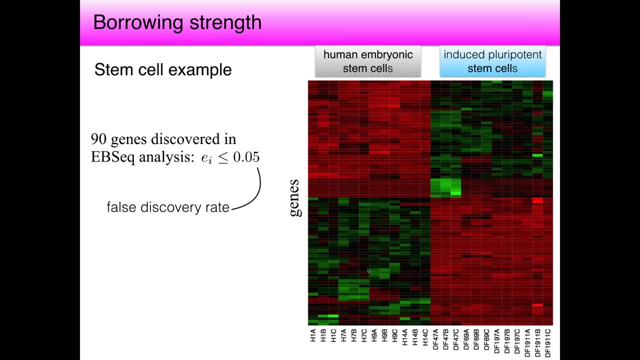 So these are posterior probabilities calculated in the model and there's a bunch of nifty formulas that you can work out for those probabilities. in the case that's considered, This just shows in a stem cell example how it would deploy where there's two conditions. 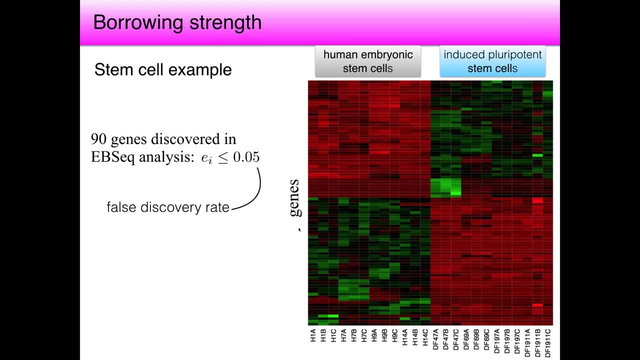 human embryonic stem cells induced pluripotent stem cells, different genes on this axis. These genes were discovered by the EBSIG analysis, So 5% FDR And there's some nice features about that, about power and robustness that other methods 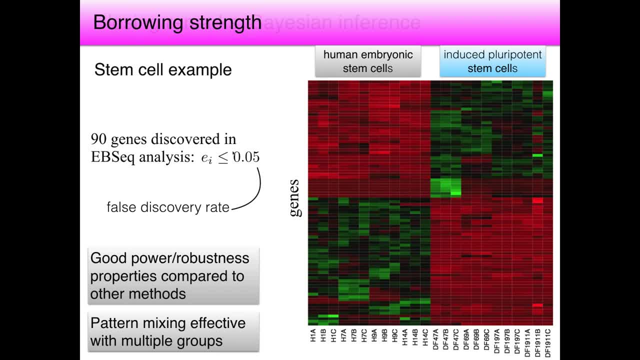 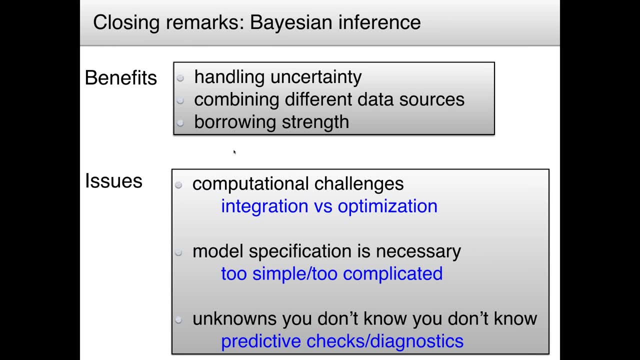 don't have such good properties on. That's a pretty quick summary of that. I want to just go to my final couple of slides on closing remarks, And I appreciate your attention. Benefits of Bayesian analysis: handling uncertainty, as I've tried to describe with the flu problem. 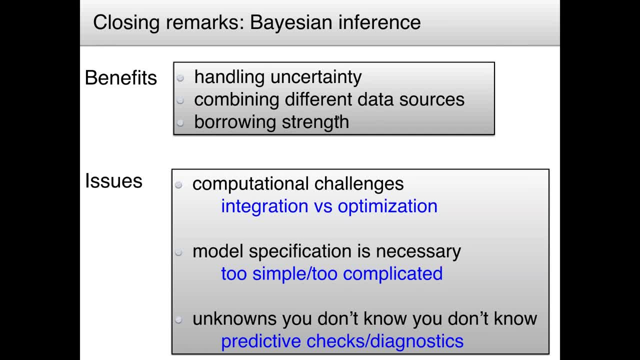 where you've got a whole bunch of things you don't know and you've got a marginal posterior structure. Combining different sources of information, of data. Bayes is natural for that, using the rules of probability Borrowing strength when you have many related but separate problems and how you can use 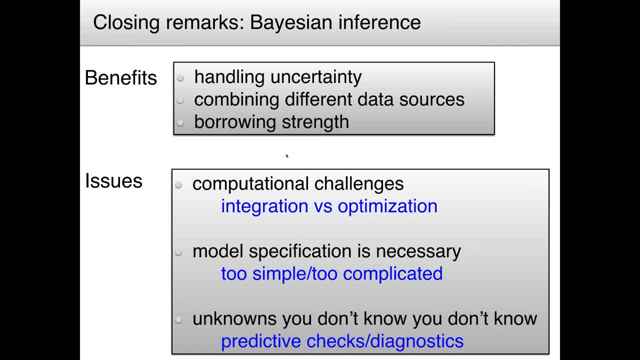 a collection of those to improve their statistical properties. There's a whole bunch of issues. There's computational challenges where a lot of learning- statistical machine learning procedures involve optimization. Bayesian procedures use a lot of integration. So there's some different issues that come up and there's a lot of challenges. data- 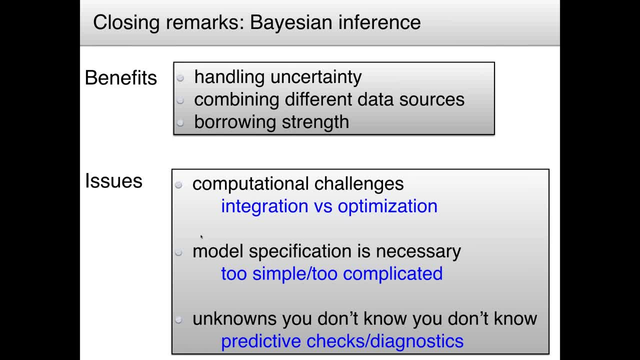 science challenges there. A big issue, Which I think is something that we're going to talk about in a little bit. We're going to talk a little bit about data science. This is something we all need to think about as we do this is that this is all built on. 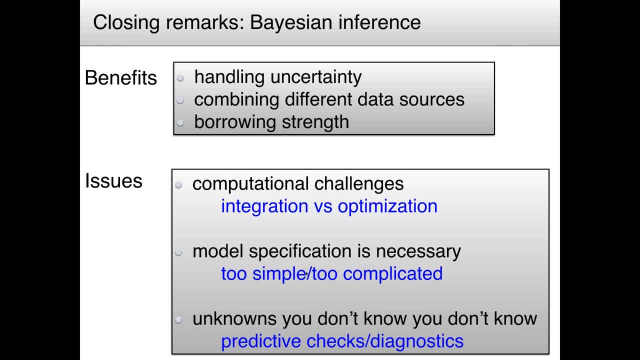 model specifications, And you can make mistakes. when you specify a probability model, The specification might be too simple. If it's too simple, you're not going to learn much new compared to some simple procedure. If it's too complicated, well, you risk all kinds of things. 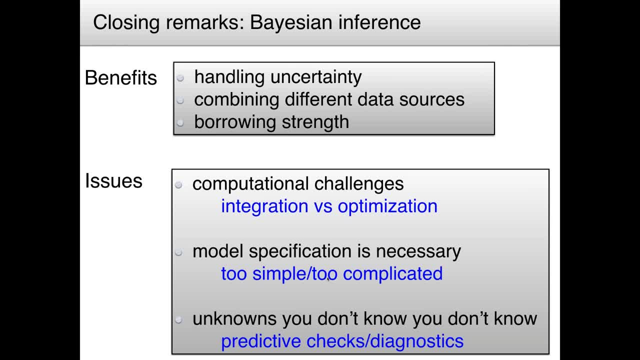 You risk making mistakes in the deployment of it. You risk that it doesn't respect the properties of the data sufficiently well. There's risks associated, And then the question, in any given situation, of the risks of making a screwy model specification: do they outweigh the benefits of improved power or improved sensitivity? 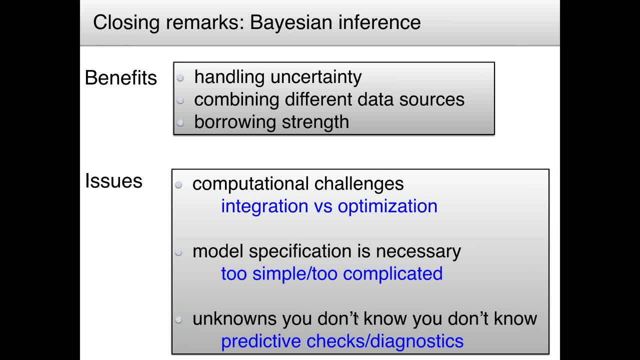 And then finally- this is last, I'll say- the unknowns you don't know. you don't know. Bayes is all about unknowns and knowns and a joint probability distribution over all those things Worried of the priors, the probability distribution of the things that you don't know. and then 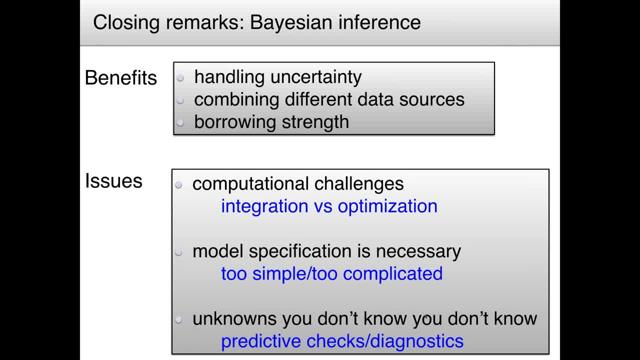 the likelihood, That's the probability of the data that you'll get to know, conditional on what you don't know, And you work out a posterior distribution of what you don't know given what you know. Except, it doesn't work if one of the you can't put a prior down on something you don't. 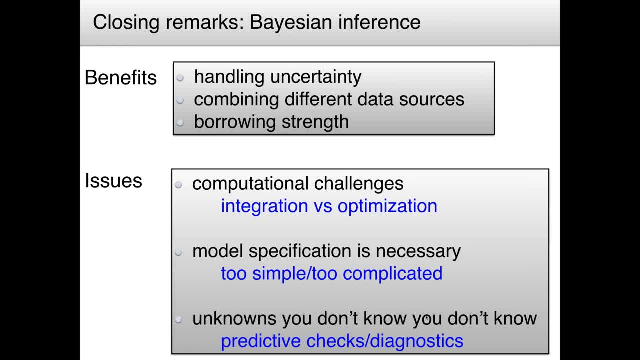 know. if you don't know that, you don't know it, And this is a fundamental issue that we have to deal with. The way it's dealt with in practice is essentially through diagnostic procedures. Obviously, all analyses are facing this thing, But we have to be upfront about it. 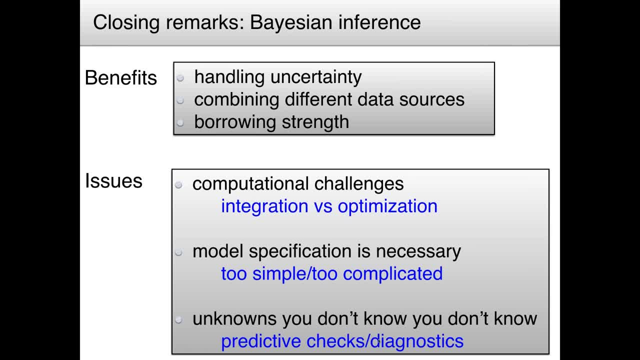 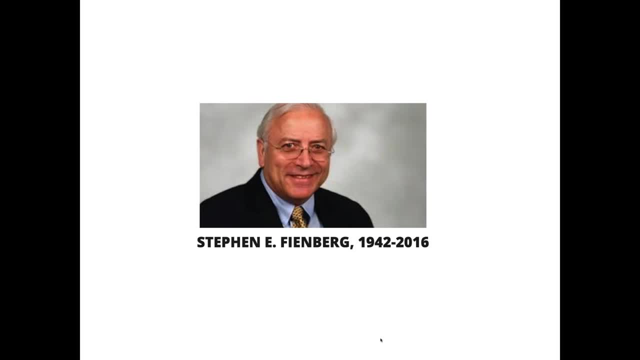 And so any model-based calculations we ever attempt to do, we need to accompany them predictive checks and diagnostics to make sure that we're not really fooling ourselves. I just want to end by dedicating this short lecture to Steve Feinberg, who passed away. 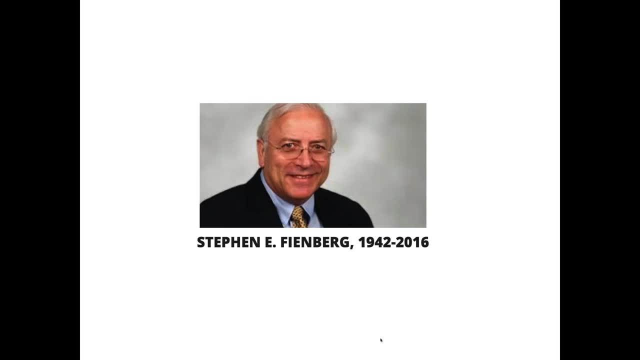 too soon last year. He was a tremendous figure, had done tons of things for the field of statistics generally and data science and Bayesian analysis, And he had a positive impact on lots of people's careers and I want to thank him for his contributions. 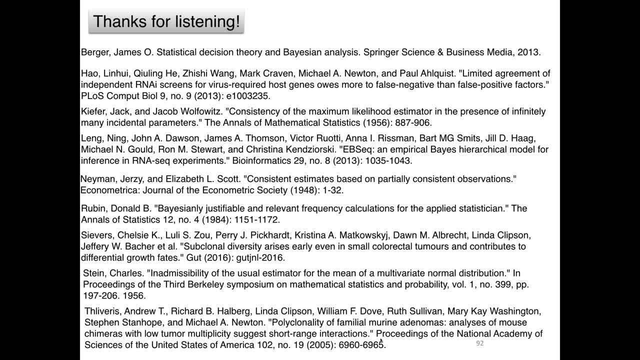 And then I just want to say thanks again to you all for listening, And I know it was quick, but the slides are available for you to look over, And here are some papers that I cited during. So thanks very much. Thanks, Michael. 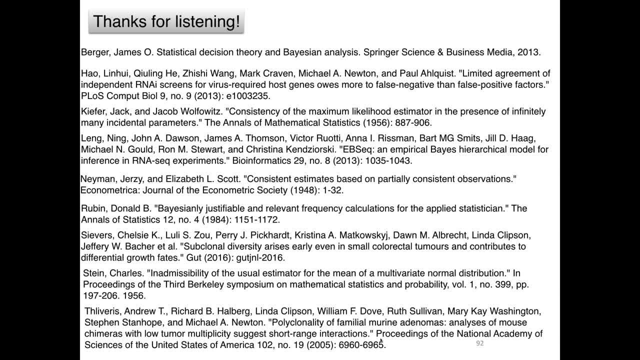 That was a great overview of Bayesian inference And you covered a lot of ground in a very short amount of time And I appreciate it. What a great job you did, explaining a lot of the more challenging concepts in this space. We have time for one quick question which is somewhat linked to the last point that 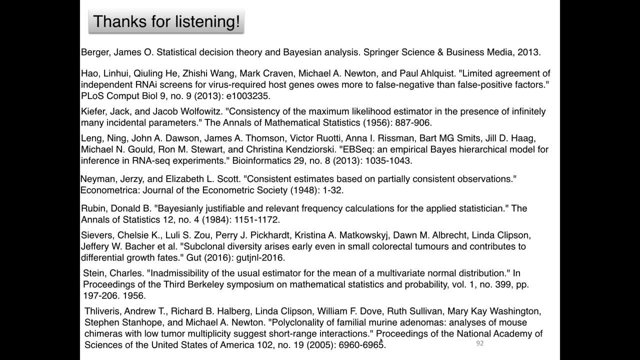 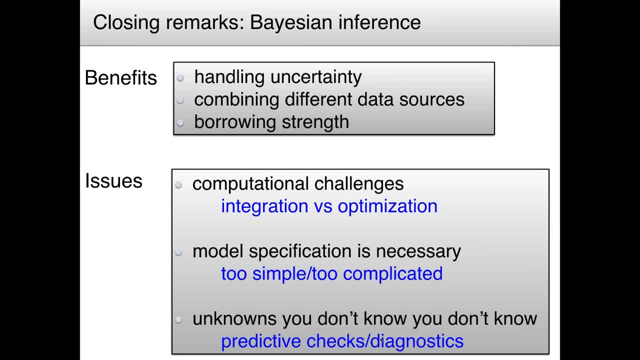 you brought up about unknowns, And I guess the challenge that we have a lot of times when we're dealing with data sets is one of both missingness and sparseness, And so I don't know if there are any new techniques that you could comment on. 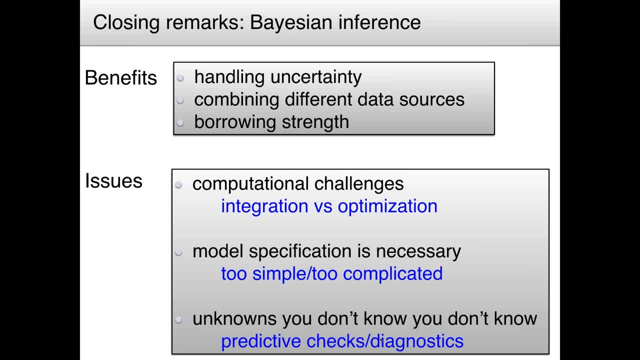 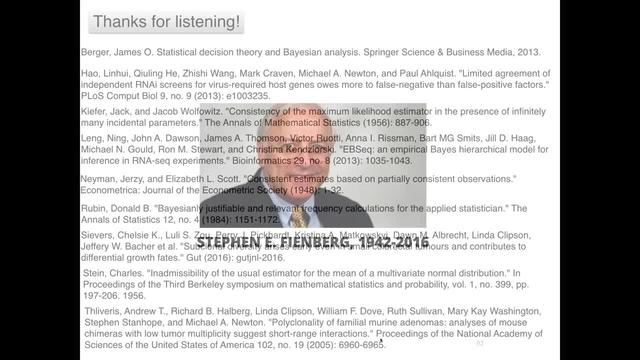 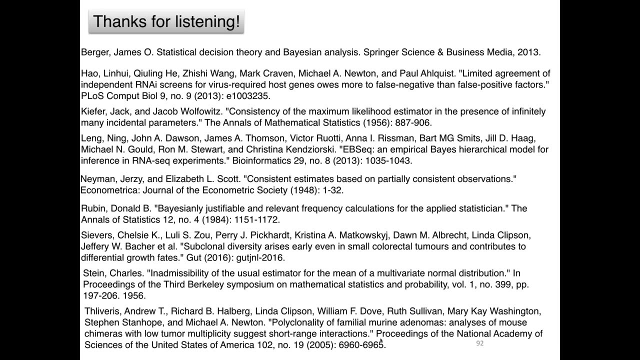 It's a great question And I think I'm going to go back to what you said earlier in terms of, from the Bayesian perspective, of how to deal with those two well, very separate issues, but if there are recommendations or suggestions you could make in that regard. 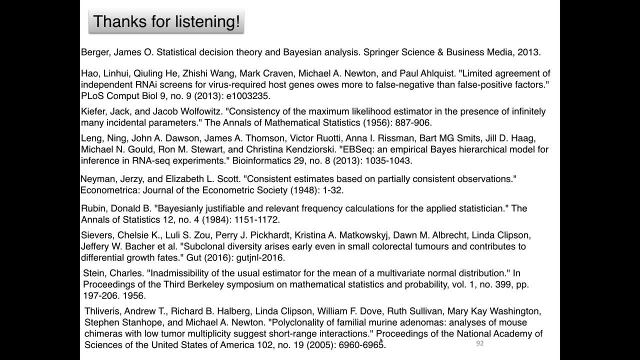 Well, I gather. next week, I think, Lance Waller is going to be talking about missingness, So I'm sure he'll have more useful things to say about the first issue, about missingness. But you're right, I mean very often. 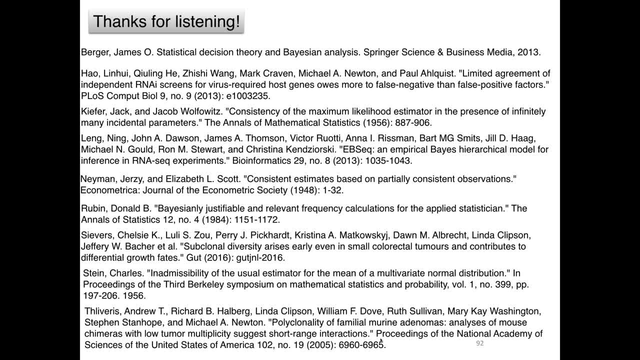 I think the way that we deal with it is in a kind of a gray zone where there's really a lot of stuff you don't have, that you would like to have, And while that's a challenge, it's also a bit of an opportunity. 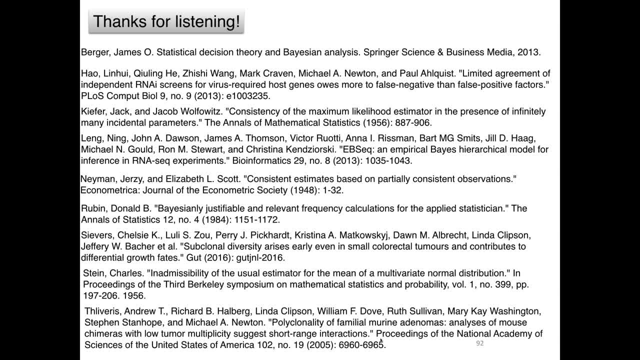 It's like: what else are you going to do if the Bayesian strategy provides a sort of general approach And then there's a lot of liberty that you have in terms of how you approach it, And what you do depends so much on the context of the situation. 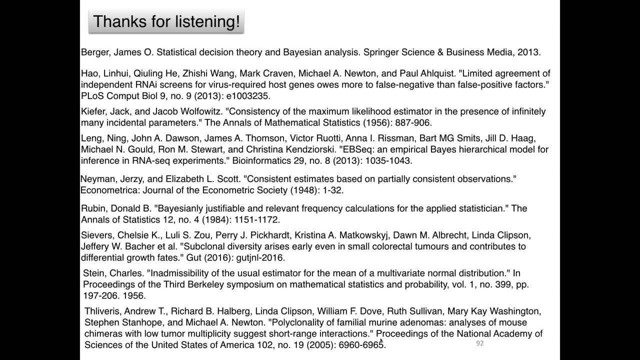 Exactly what is the relevant information that you have, or the relevant information that you don't know? How can you usefully summarize the data down? What parts of data should you not have summarized away? So I think you need to sit yourself in this kind of a Goldilocks scenario where the model 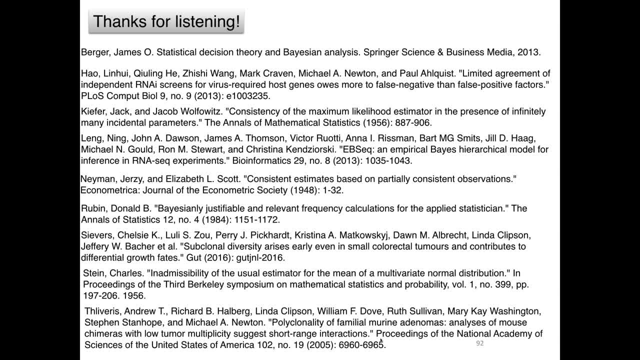 might be too simple, the model might be too complicated. if the problem that you're addressing is sufficiently important and you have enough time to think hard about it, then you could try something like this, And essentially, what you need to do is write down some kind of probability structure for 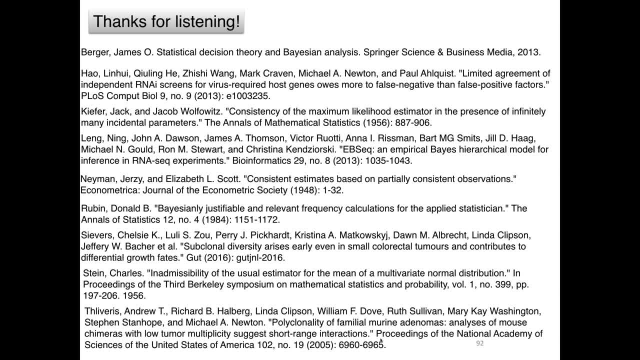 all those things that you don't know And exactly what that would look like. I mean, that depends very much on the context, doesn't it? I would say that in some classical probability models, like regression models, where sparsity is an issue that's very often discussed, with these penalized estimation procedures and 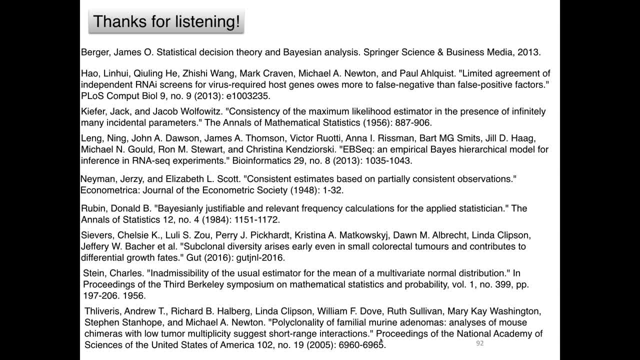 all that, I think that, more fully, Bayesian tools for understanding the good procedures in those situations have recently been, I think, discovered and debated. So there's a group at Warwick that's doing a lot with that. There's Nick Paulson's group in Chicago that's done a bunch of interesting things.